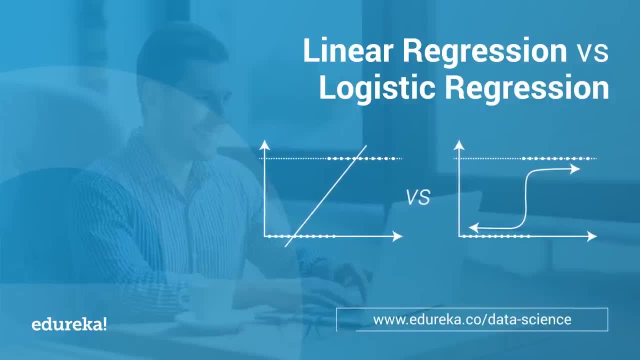 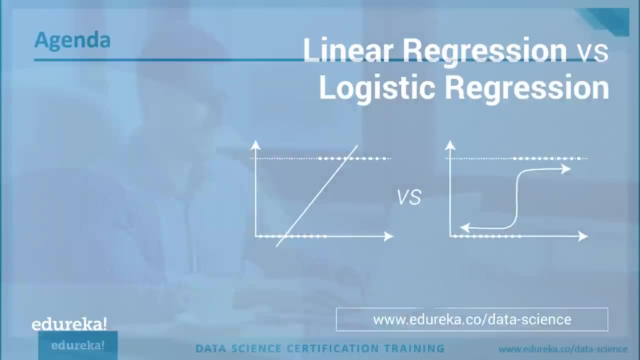 machine learning algorithms. there is still a lot of confusion between them, and today we'll compare the two and see how they work. So, without any further delay, let's take a look at today's agenda. We're going to begin the session with a discussion on the various types of machine learning. 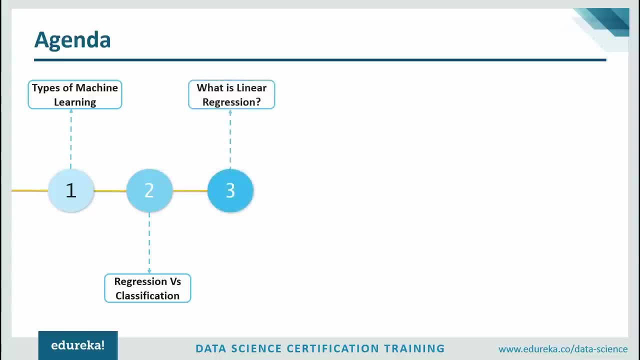 Next we'll see what exactly linear regression is and how it works. After that we'll move on and discuss about logistic regression. Then we look at a linear regression use case and a logistic regression use case. Finally, we'll end the session by comparing linear regression. 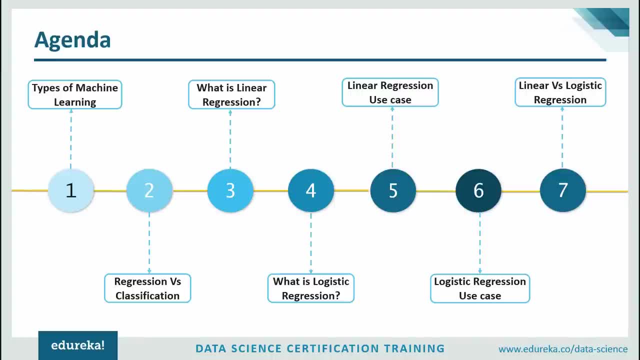 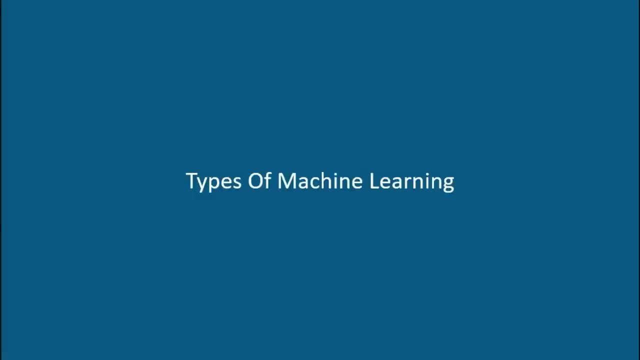 and logistic regression. So, guys, let's take a look at today's first topic Now, before I begin with the types of machine learning. if any of you guys are interested in machine learning or want to learn more about machine learning, I'm going to leave a link in the description. You all can. 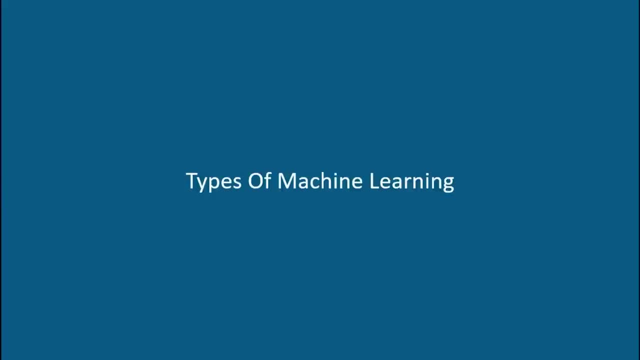 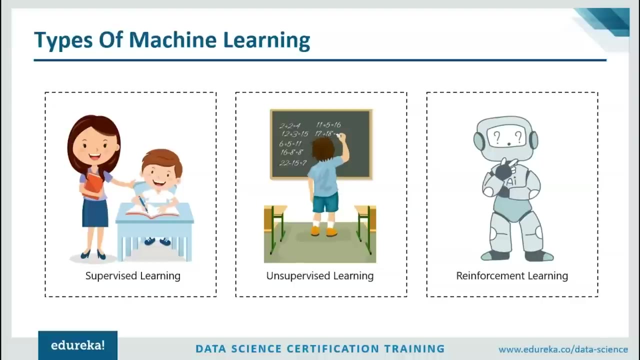 check out that video and then probably get back to this one. Alright, so let's begin with the types of machine learning. So, guys, first we have supervised learning. In this type of learning, the machine learns under guidance. So, if you remember, at school our teachers guided. 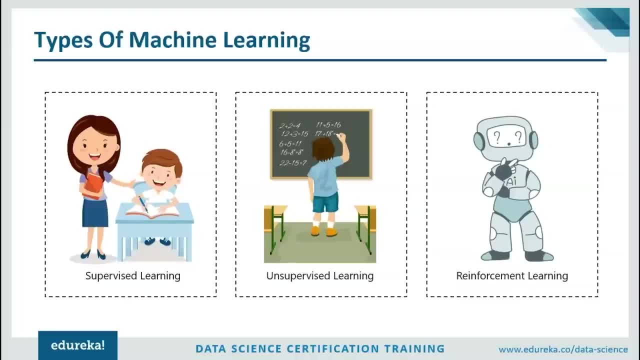 us and taught us Similarly in supervised learning, machines learn by feeding them label data and explicitly telling them: hey, this is the input and this is how the output must look. The teacher, in this case, is the training data. Next up, we have unsupervised learning Now here. 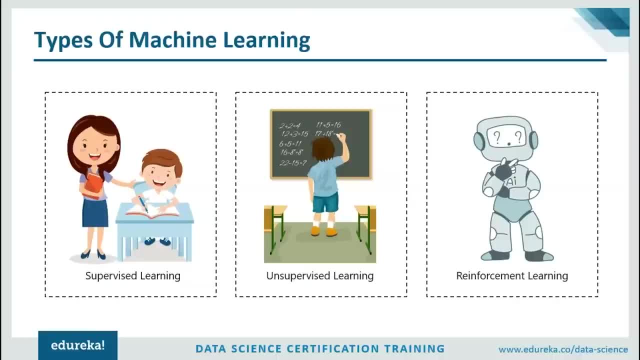 the data is not labeled, There is no guide at all, The machine has to figure out the data set given and it must find hidden patterns in order to make predictions about the output. So an example of unsupervised learning is an adult like you and me. 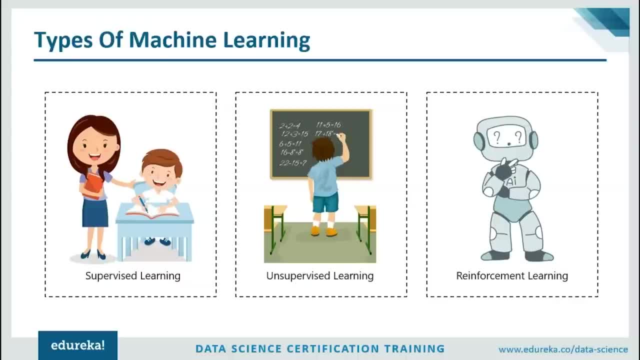 We don't need a guide to help us with our daily activities, right? We figure things out on our own without any supervision. Now, finally, we have reinforcement learning. So let's say that you were dropped off at an isolated island. So, guys, what would you do Initially? you would panic and 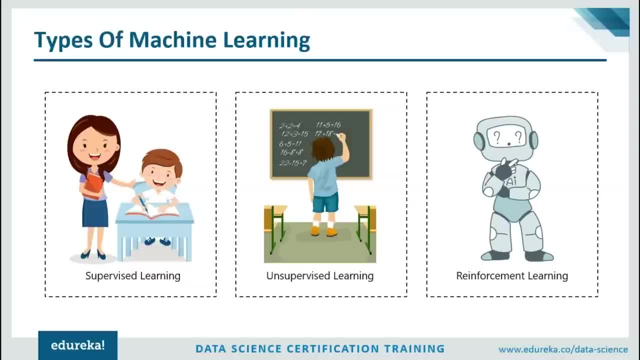 you'd be unsure of what to do, where to get food from, how to live and so on. But after a while you will have to adapt. You have to learn how to live in the island, adapt to the changing climates, learn what to eat and what not to eat. So, basically, 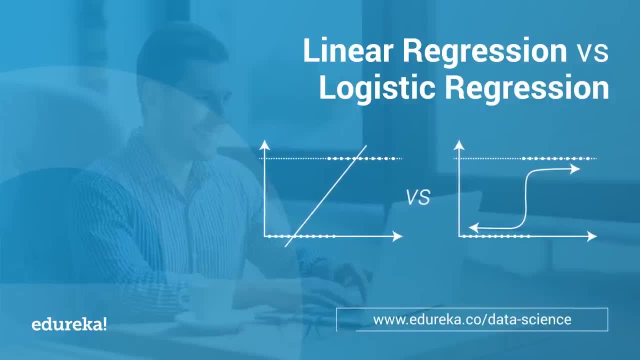 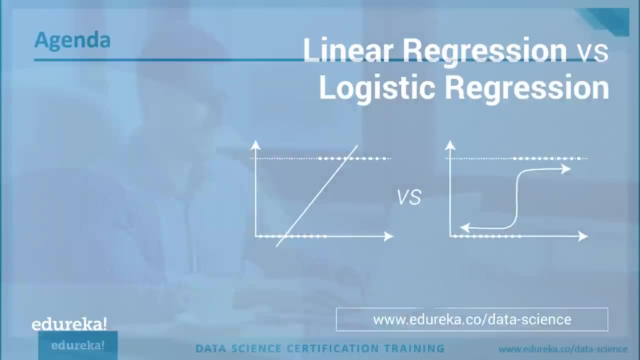 machine learning algorithms. there is still a lot of confusion between them, and today we'll compare the two and see how they work. So, without any further delay, let's take a look at today's agenda. We're going to begin the session with a discussion on the various types of machine learning. 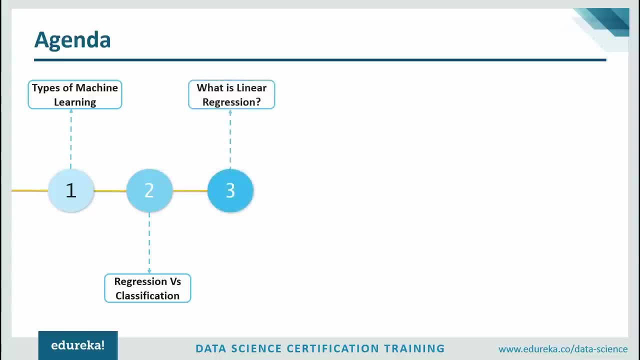 Next we'll see what exactly linear regression is and how it works. After that we'll move on and discuss about logistic regression. Then we look at a linear regression use case and a logistic regression use case. Finally, we'll end the session by comparing linear regression. 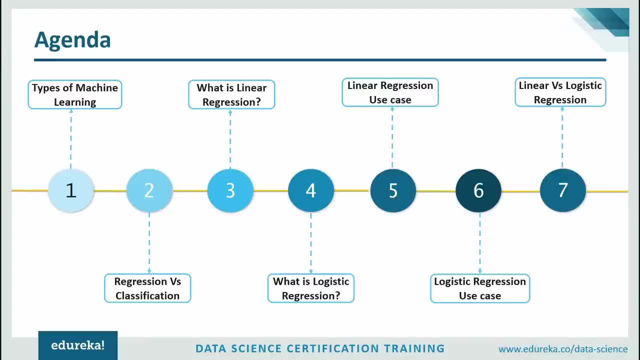 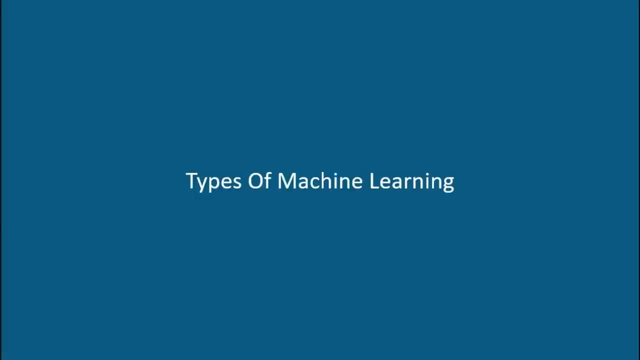 and logistic regression. So, guys, let's take a look at today's first topic Now, before I begin with the types of machine learning. if any of you guys are interested in machine learning or want to learn more about machine learning, I'm going to leave a link in the description You all can check. 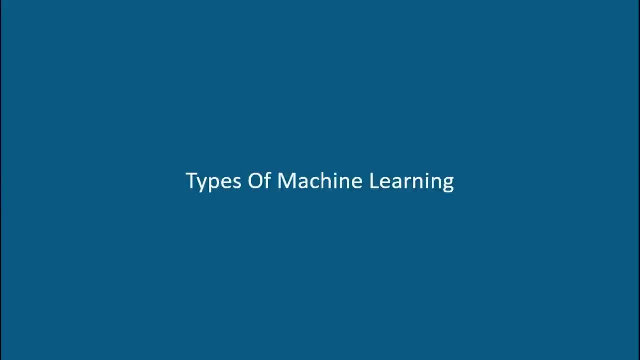 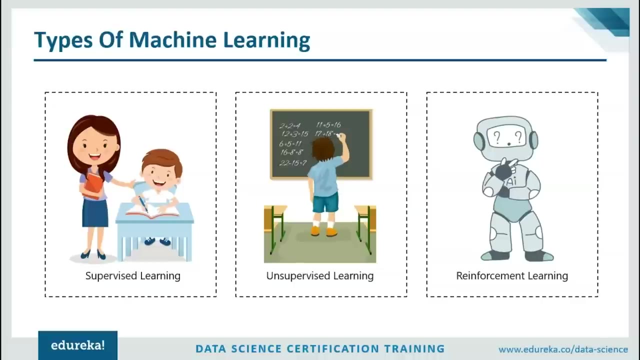 out that video and then probably get back to this one. All right, so let's begin with the types of machine learning. So, guys, first we have supervised learning. In this type of learning, the machine learns under guidance. So, if you remember, at school our teachers guided us on how to learn. 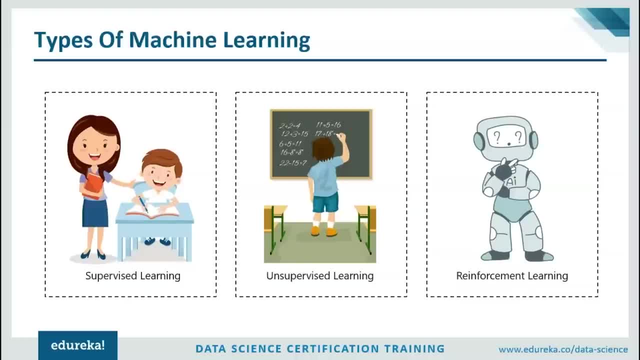 and taught us Similarly in supervised learning, machines learn by feeding them label data and explicitly telling them: hey, this is the input and this is how the output must look. The teacher in this case is the training data. Next up, we have unsupervised learning. Now, here, the data is not. 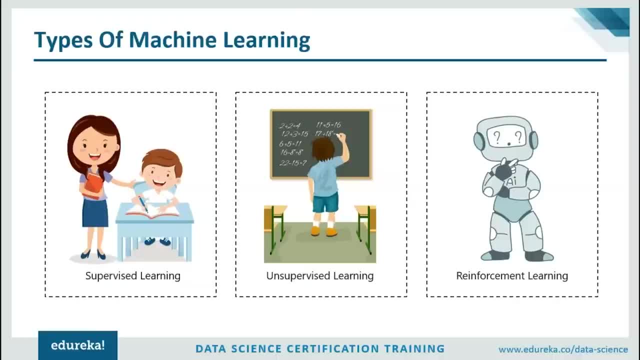 labeled, There is no guide at all. The machine has to figure out the data set given and it must find hidden patterns in order to make predictions about the output. So an example of unsupervised learning is an adult like you and me. We don't need a guide to help us with our daily activities. right, We figure things out on our own. 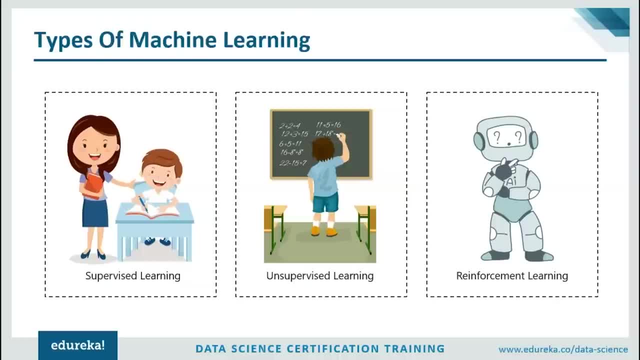 without any supervision. Now, finally, we have reinforcement learning. So let's say that you were dropped off at an isolated island. So, guys, what would you do? Initially you would panic and you'd be unsure of what to do, where to get food from, how to live, and so on. But after a while you will. 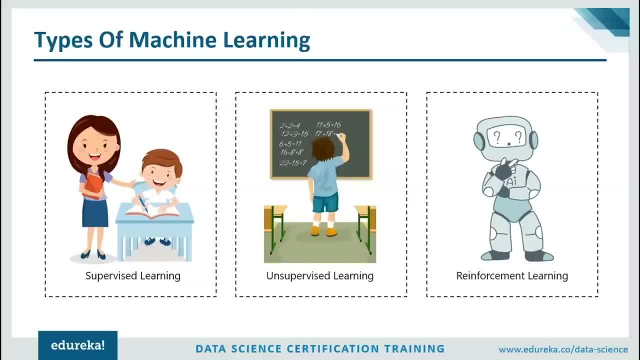 have to adapt. You have to learn how to live in the island, adapt to the changing climates, learn what to eat and what not to eat. So, basically, what you're doing is you're going to learn how to live in the island. What you're doing is you're following the hit and trial concept, because you're 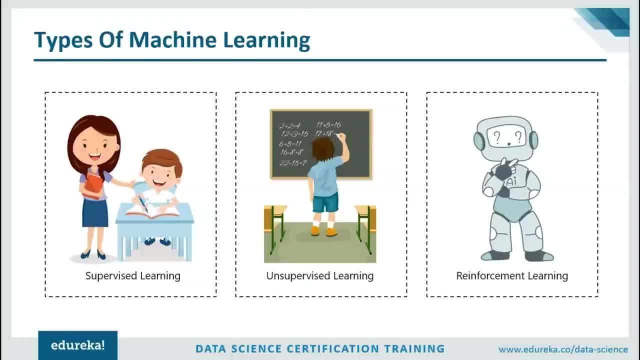 what you're doing is you're following the hit and trial concept, because you're new to the surrounding and the only way for you to learn is experience and then learn from your experience. So this is what reinforcement learning is about. It is a learning method wherein an agent interacts with 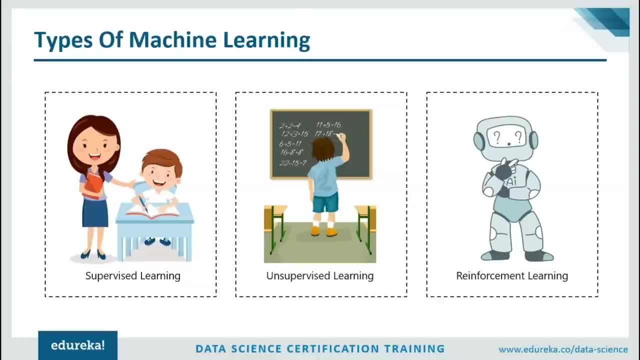 its environment by producing some actions, and it discovers errors or rewards. So, guys, this was a brief discussion about the types of machine learning. Now let's move ahead and look at the different types of supervised learning problems. All right, So, like I said, we have unsupervised learning. 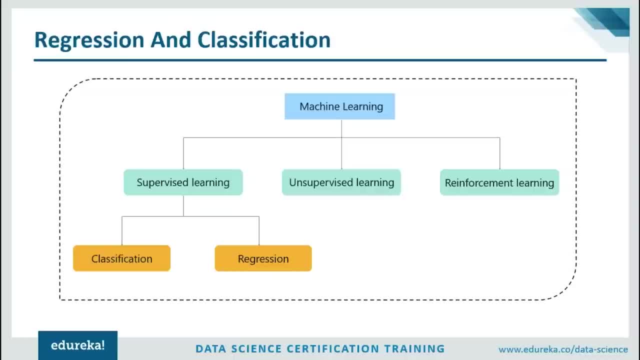 As I said earlier, machine learning has three types of learnings. Okay, it's supervised learning, unsupervised learning and reinforcement learning. now, under supervised learning, We have two classes of problems. Okay, so there are two problems that we can deal with. one is a classification problem. 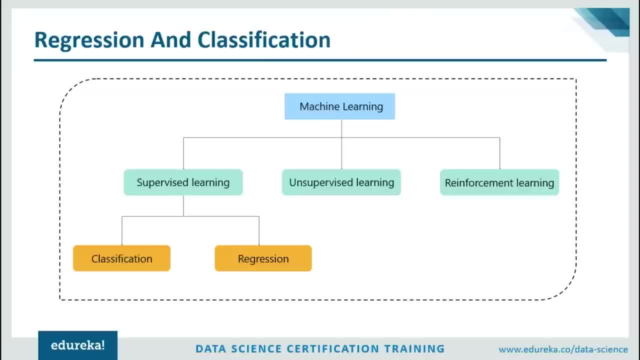 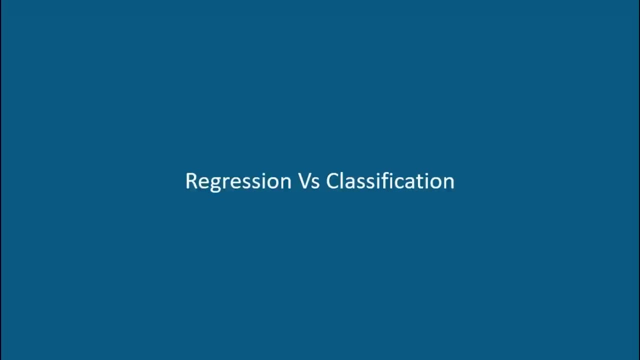 and the other is a regression problem. So here we'll be focusing on supervised learning itself, because our linear regression and our logistic regression are actually supervised learning algorithms. Okay, Now, before we start discussing about linear and logistic regression, let's try to differentiate between classification problems and regression problems. So, guys there, 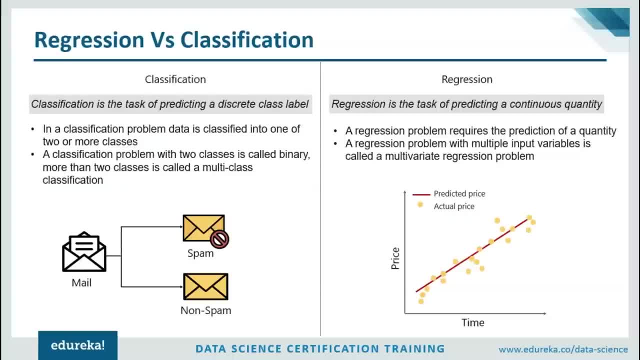 is an important difference between classification and regression problems. Basically, classification is about predicting a label and regression is about predicting a quantity. Okay, So let's say that you want to classify your emails into two groups. So, basically, what we'll be doing is we'll be labeling. 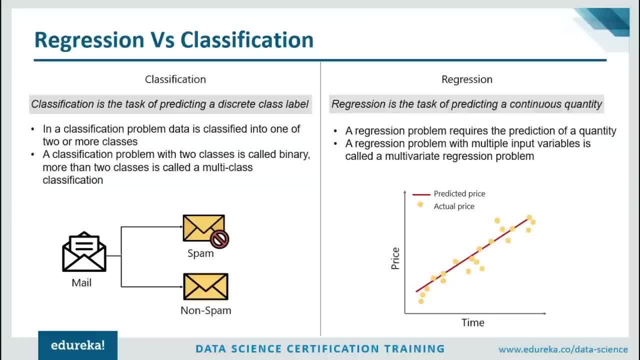 our mails as spam and non-spam mails. Okay, So for this kind of problem, where we have to assign our input data Into different classes, we make use of classification algorithms. Now, under classification, we have two types. We have binary classification and multi-class classification. Now the example. 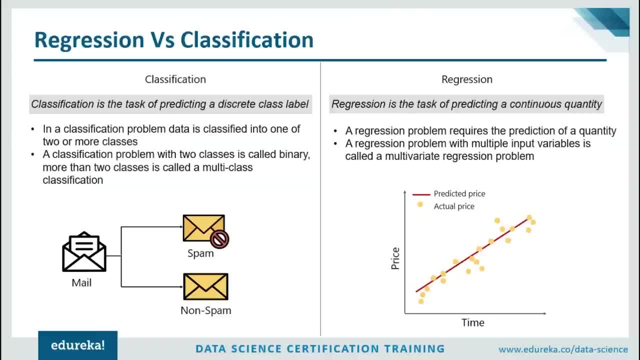 that I gave earlier about classifying emails as spam and non-spam is of binary type. Now, this is because here we are classifying mails into only two classes: spam and non-spam. But let's say that we want to classify mails into three classes: one containing spam messages. second, one containing 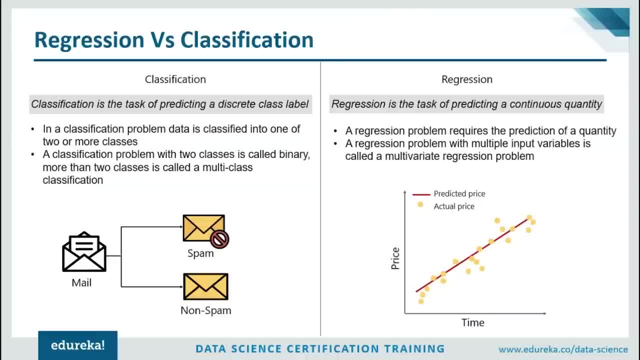 non-spam messages And third one, let's say, containing drugs. So here what we're doing is we're classifying mails into more than two classes. This is exactly what multi-class classification means. now, one more thing to note here is that it is common for classification models to predict a continuous value. 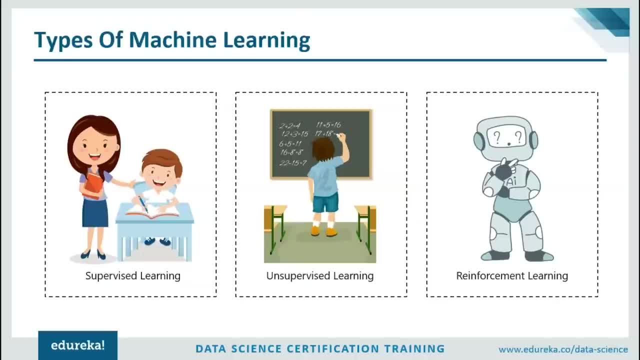 new to the surrounding, and the only way for you to learn is experience and then learn from your experience. So this is what reinforcement learning is about. It is a learning method wherein an agent interacts with its environment by producing some actions and it discovers errors or rewards. 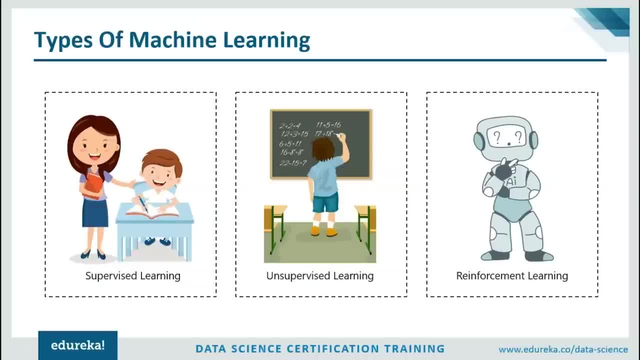 So, guys, this was a brief discussion about the types of machine learning. Now let's move ahead and look at the different types of supervised learning problems. All right, So, like I said earlier, we have unsupervised learning, We have unsupervised learning. We have unsupervised learning. 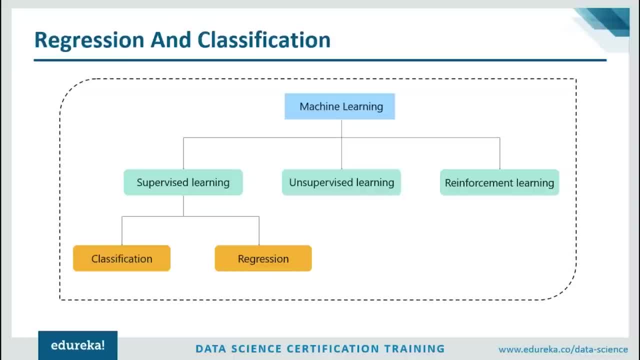 Machine learning has three types of learnings. Okay, it's supervised learning, unsupervised learning and reinforcement learning. now, under supervised learning, We have two classes of problems. Okay, so there are two problems that we can deal with. one is a classification problem and the other 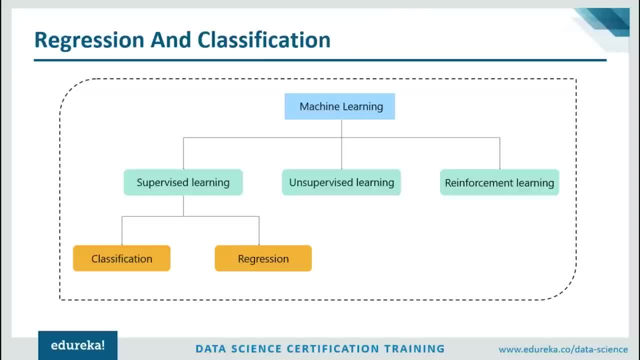 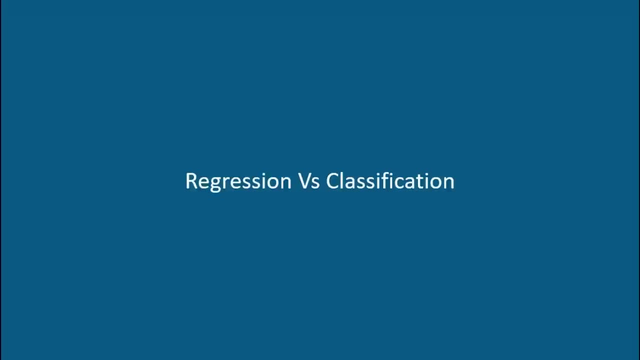 is a regression problem. So here we'll be focusing on supervised learning itself, because our linear regression and our logistic regression are actually supervised learning algorithms. Okay, Now, before we start discussing about linear and logistic regression, let's try to differentiate between classification problems and regression problems. 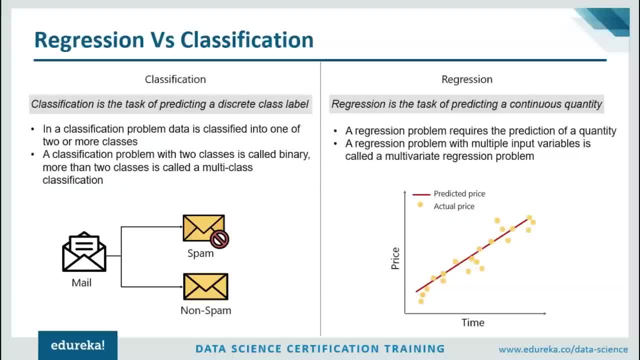 So, guys, there is an important difference between classification and regression problems. Basically, classification is about predicting a label and regression is about predicting a quantity. Okay, So let's say that you want to classify your emails into two groups. So basically, what we'll be doing is we'll be labeling our males as spam and non-spam males. 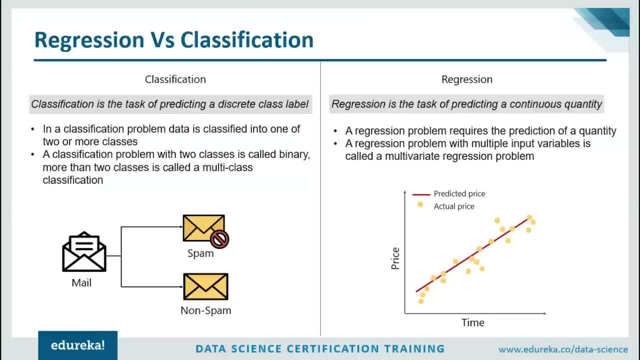 Okay. So for this kind of problem, where we have to assign our input data into different classes, We make use of classification algorithms. now, under classification, We have two types. We have binary classification and multi-class classification. Now, the example that I gave earlier about classifying emails as spam and non-spam is of binary type. 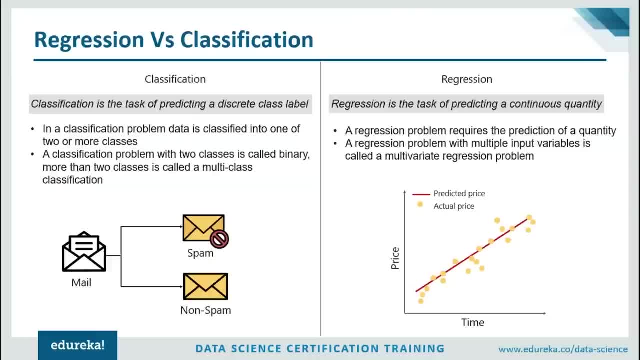 Now, this is because here we are classifying males into only two classes: spam and non-spam. but let's say that we want to classify males into three classes: one containing spam messages, second one containing non-spam messages And third one, let's say, containing drafts. 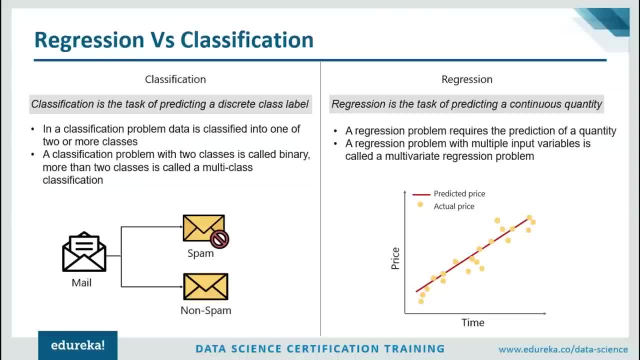 So here what we're doing is we're classifying males into more than two classes. This is exactly what multi-class classification means. now, one more thing to note here is that it is common for classification models to predict a continuous value, but this continuous value actually represents the probability. 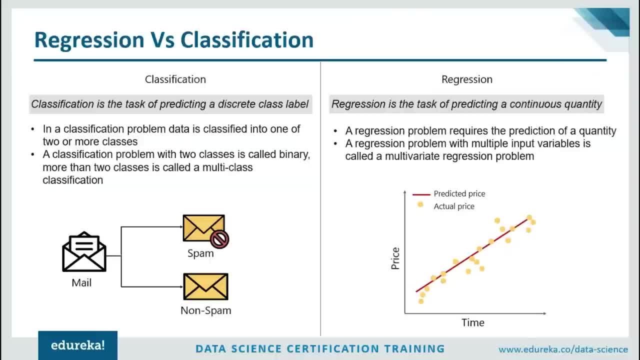 of a given data point belonging to each output class. So always the end result in a classification problem is going to be a label or a class. Now let's discuss about regression. So, guys, regression is used to predict a continuous quantity. Now, when I say a continuous quantity, 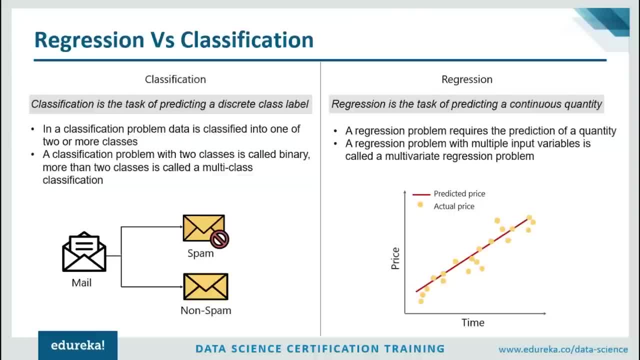 it's basically a continuous variable. a continuous variable is a variable that has infinite number of possibilities. Now, for example, a person's weight. someone could weigh 180 pounds, or they could weigh 180.10 pounds or 180.110 pounds. Okay, so the number of possibilities for weight is limitless. 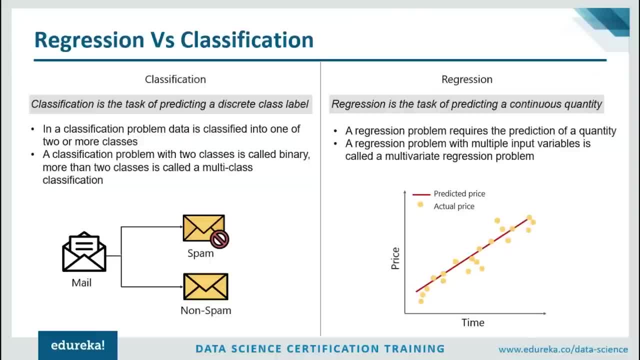 and this is exactly what a continuous variable It is. so, guys, regression is a predictive analysis used to predict continuous variables. So in regression, you don't have to label data into different classes, All right. instead, you have to predict a final outcome. 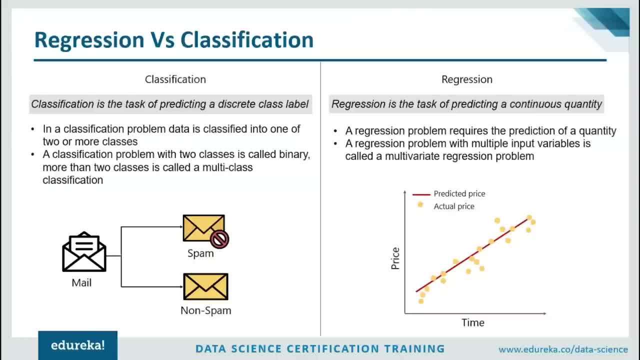 Like, let's say, you want to predict the price of a stock over a period of time. for such a problem You can make use of regression by studying the relation between the dependent variable, which is basically your stock price, and the independent variable, which is the time. so, guys, I was a brief summary. 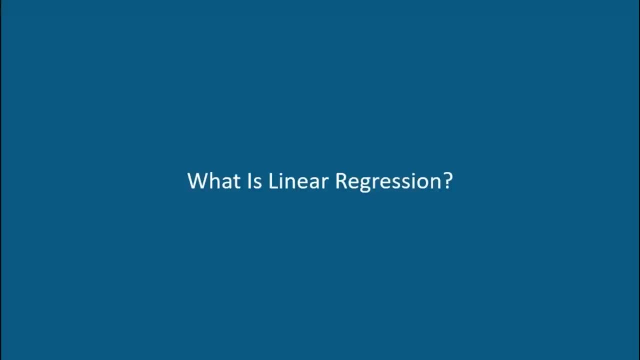 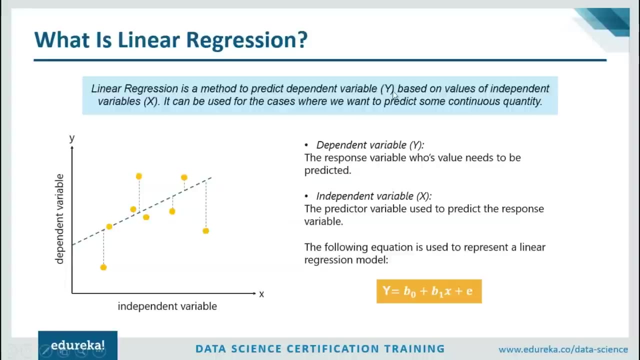 Of regression and classification. now let's move ahead and see what exactly linear regression is. So, guys, linear regression is a method to predict a dependent variable Y based on values of independent variables X. So in the previous example where I discuss about the stock price, the dependent variable, 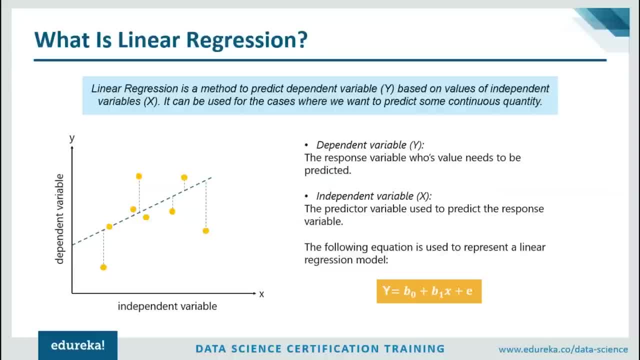 is a stock price, since the price of a stock depends and varies over a period of time, correct. So, because the stock price is dependent on some other variable, It's known as a dependent variable. and one more important thing to note here is that the dependent variable 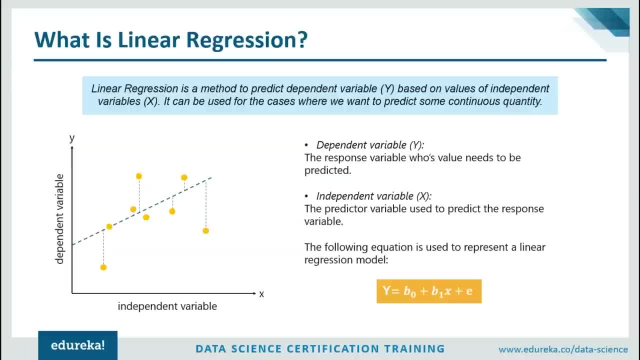 for a linear regression model is always continuous. now, guys, This is a very important point, because this is one of the major attributes of a linear regression model. So the dependent variable for a linear regression model is always continuous. So here the price of a stock is continuous. 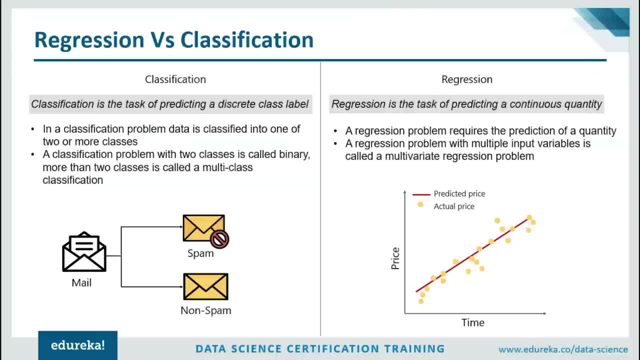 but this continuous value actually represents the probability of a given data point belonging to each output class. So always, the end result in a classification problem is going to be a label or a class. Now let's discuss about regression. So, guys, regression is used to predict a continuous quantity. 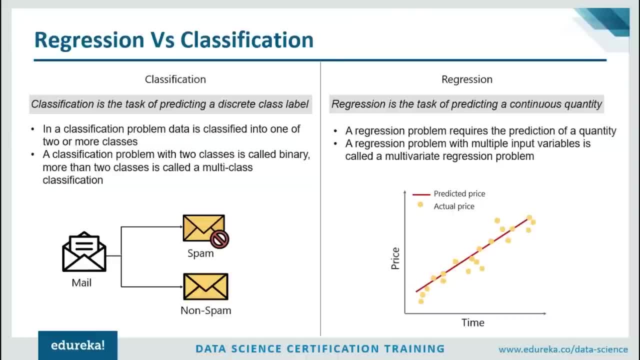 Now, when I say a continuous quantity, it's basically a continuous variable. a continuous variable is a variable that has infinite number of possibilities. Now, for example, a person's weight. someone could weigh 180 pounds, or they could weigh 180.10 pounds or 180.110 pounds. 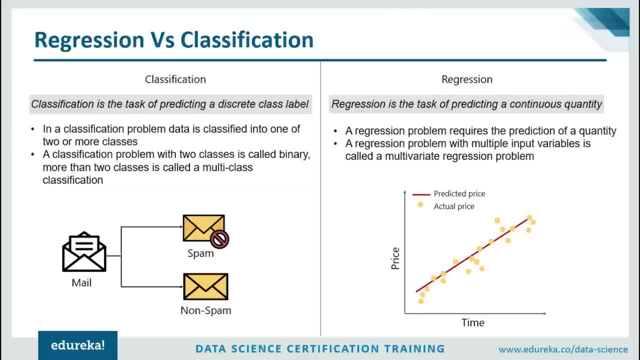 Okay, so the number of possibilities for weight is limitless, and this is exactly what a continuous weight is limitless, and this is exactly what a continuous weight is limitless, and this is exactly what a continuous variable is. so, guys, regression is a predictive analysis used to predict continuous variables. 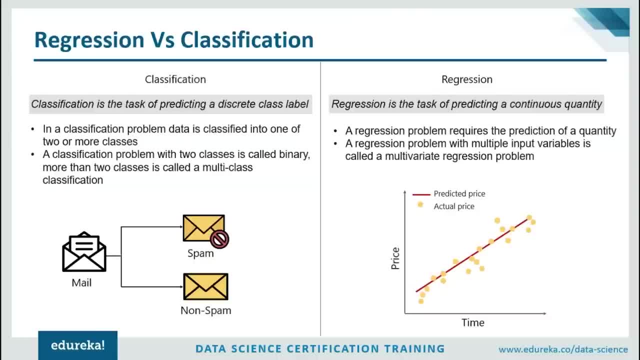 So in regression you don't have to label data into different classes, All right. instead, you have to predict a final outcome, Like, let's say, you want to predict the price of a stock over a period of time. for such a problem You can make use of regression by studying the relation between the dependent variable. 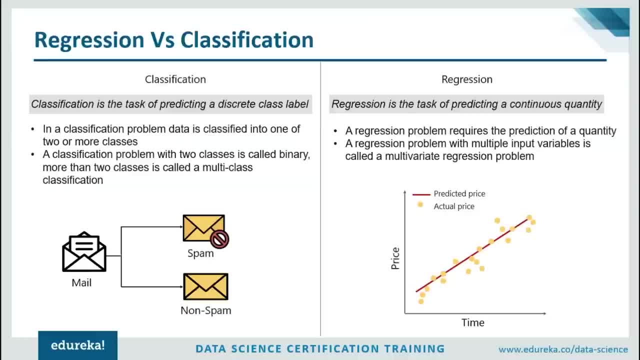 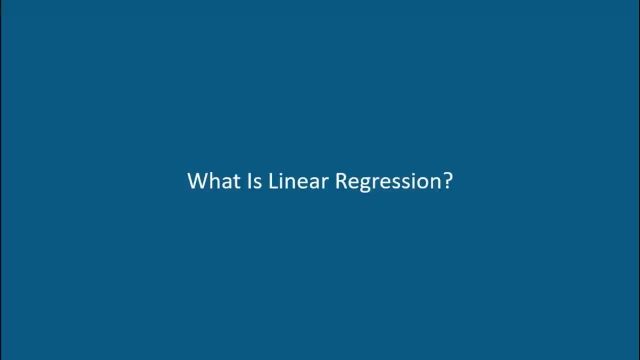 which is basically your stock price, and the independent variable, which is the time. So, guys, that was a brief summary of regression and classification. Now let's move ahead and see what exactly linear regression is. So, guys, linear regression is a method to predict a dependent variable. 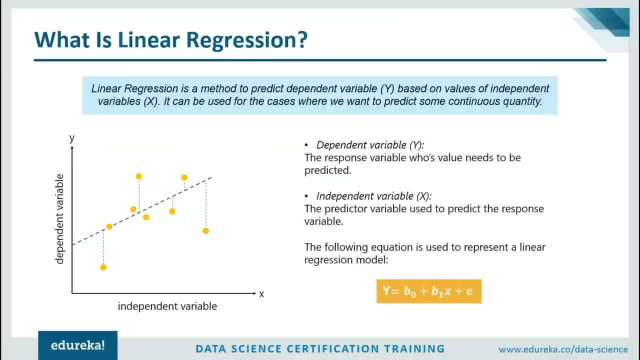 Why? based on values of independent variables X. So in the previous example, where I discuss about the stock price, the dependent variable is a stock price, since the price of a stock depends and varies over a period of time. correct? So, because the stock price is dependent. 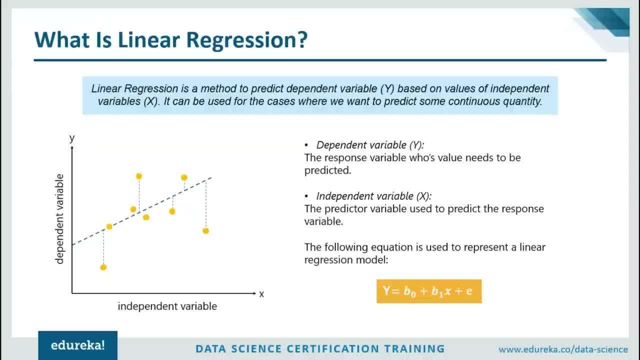 on some other variable. it's known as a dependent variable, and one more important thing to note here is that the dependent variable for a linear regression model is always continuous. Now, guys, this is a very important point, because this is one of the major attributes of a linear regression model. 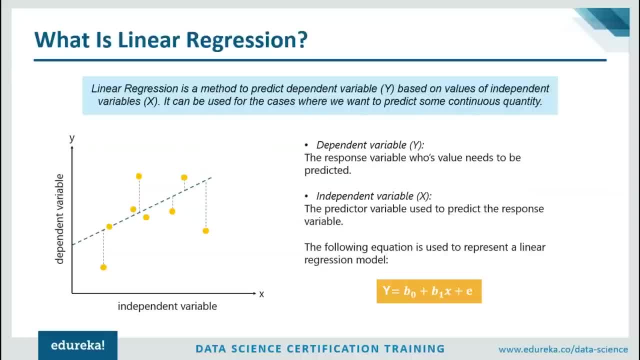 So the dependent variable for a linear regression model is always continuous. So here the price of a stock is continuous because it can have infinite possible values. All right. now, on the other hand, time is the independent variable. Okay, it can either be continuous or it can be discreet. 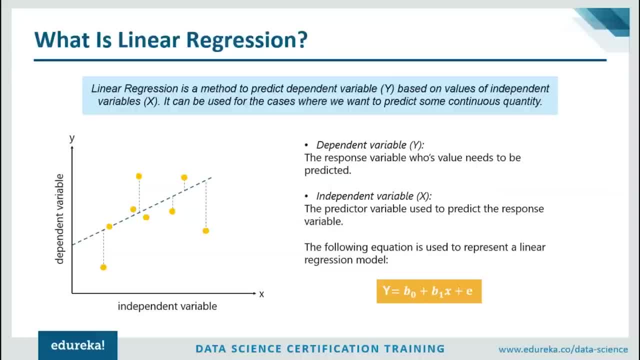 because it can have infinite possible values. All right, now, on the other hand, time is the independent variable. Okay, it can either be continuous Or it can be discrete. now this dependent variable is used to decide the value of the dependent variable. Like I mentioned earlier, the stock price can change depending. 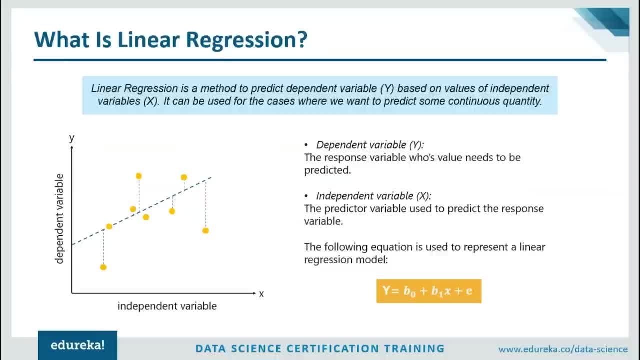 on the time. Okay, so it varies over a period of time. That's why time is considered as the independent variable. Okay, Now let's look at how a linear regression works. So first of all, we try to figure out a relationship. 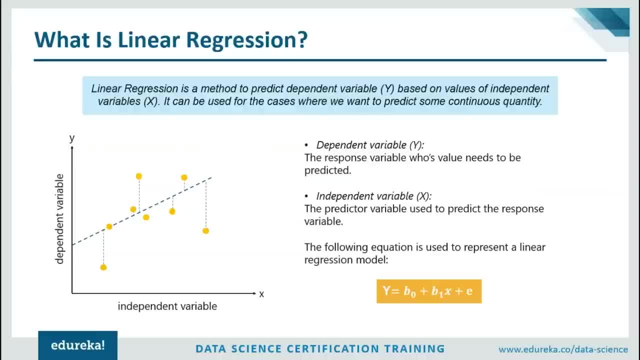 between our dependent variable and the independent variable by using a best-fitting straight line. Now, linear regression is called a simple model, because we only take two variables in this case and we try to establish a relation between them. Now the reason why linear regression is called linear. 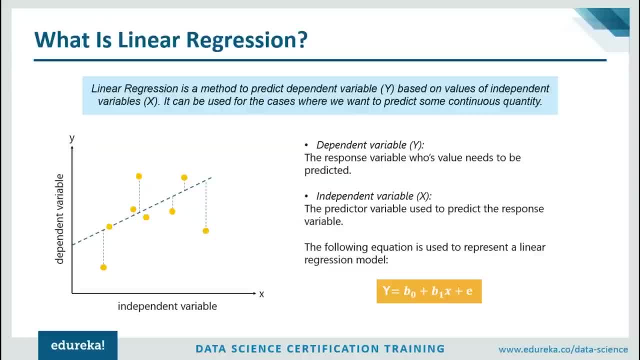 is because both the variables vary linearly with respect to each other. So basically, the stock price and the time are linearly dependent on each other. So while plotting the relationship between two variables, will be observing more of a straight line instead of a curve, because they're linearly dependent. 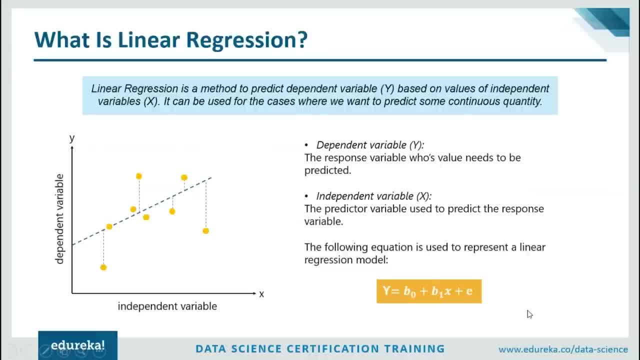 Now let's discuss the math behind linear regression. So the equation that you see over here, y is equal to B naught plus B. 1 into X plus E- is used to represent a linear regression model. So this equation is used to draw out a relation. 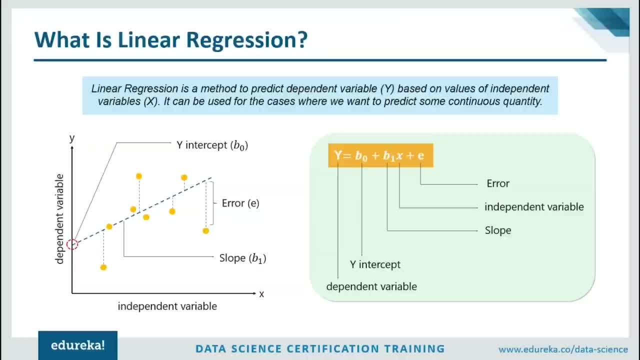 between the independent variable X and the dependent variable Y. now we all know the equation for a linear line in math, which is y is equal to MX plus C. So basically, the linear regression equation is represented along the same equation. All right, because this is a straight line. 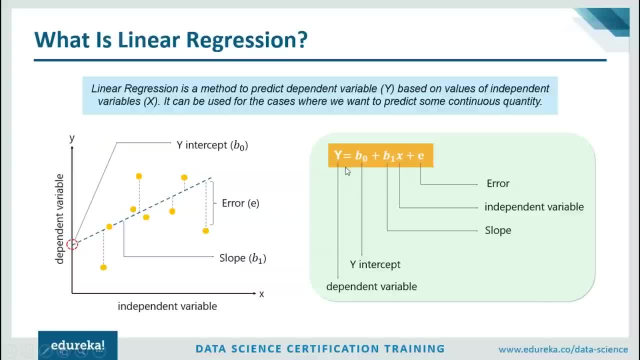 Let's break down this formula Now. y over here basically stands for the dependent variable that needs to be predicted. Okay, so maybe this is the stock price. now, B naught is basically the y-intercept, which is basically the point on this line which touches the y-axis. 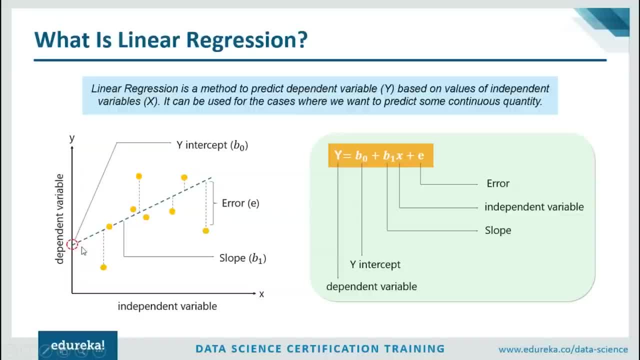 Okay, that's why it's called y-intercept. So this is our B naught over here. B 1 is the slope of this line, this linear line, and the slope can be either negative or positive depending on the relation between the dependent variable. 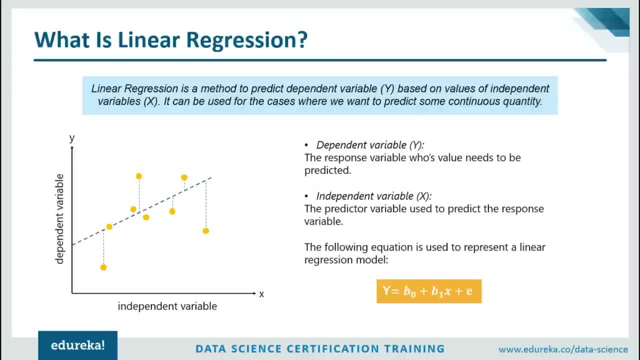 Now this dependent variable is used to decide the value of the dependent variable. Like I mentioned earlier, the stock price can change depending on the time. Okay, so it varies over a period of time. That's why time is considered as the independent variable. 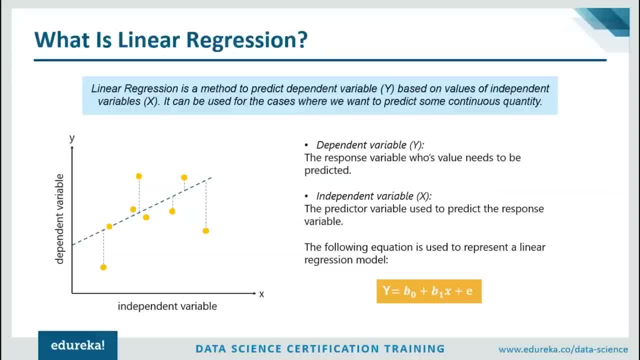 Okay, Now let's look at how a linear regression works. So first of all, we try to figure out a relationship between our dependent variable and the independent variable by using a best-fitting straight line. Now, linear regression is called a simple model. 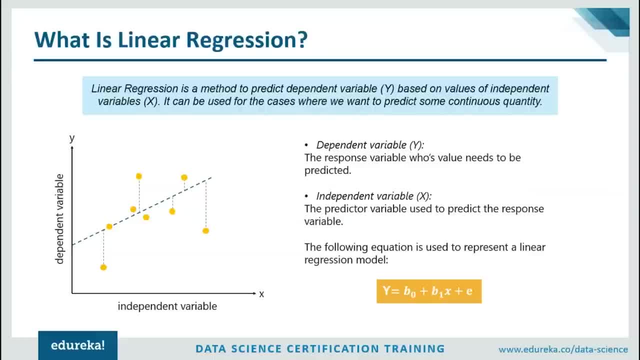 because we only take two variables in this case and we try to establish a relation between them. Now, the reason why linear regression is called linear is because both the variables vary linearly with respect to each other. So basically, the stock price and the time are linearly dependent on each other. 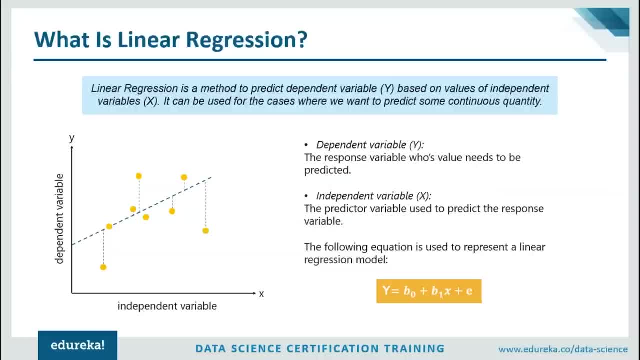 So, while plotting the relationship between two variables, will be observing more of a straight line instead of a curve, because they're linearly dependent. Now let's discuss the math behind linear regression. So the equation that you see over here, Y is equal to B, naught. 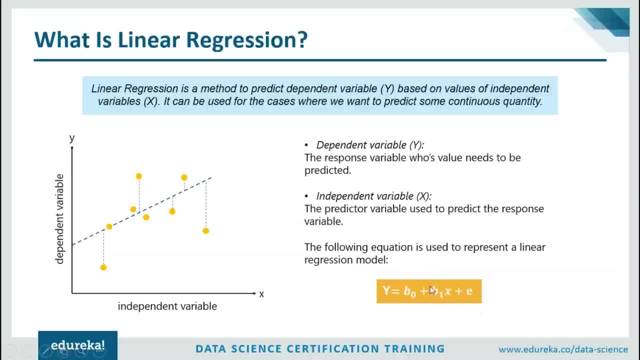 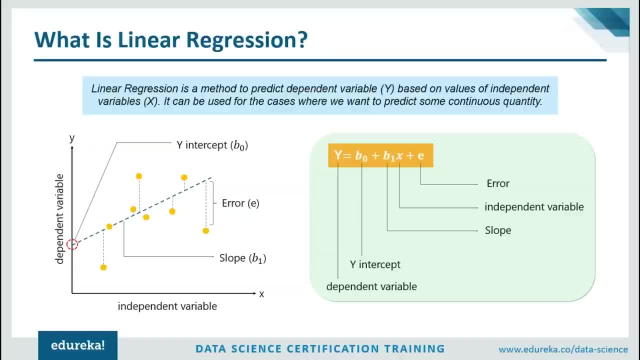 plus B, 1 into X plus E is used to represent a linear regression model. So this equation is used to draw out a relation between the independent variable X and the dependent variable Y. now we all know the equation for a linear line in math. 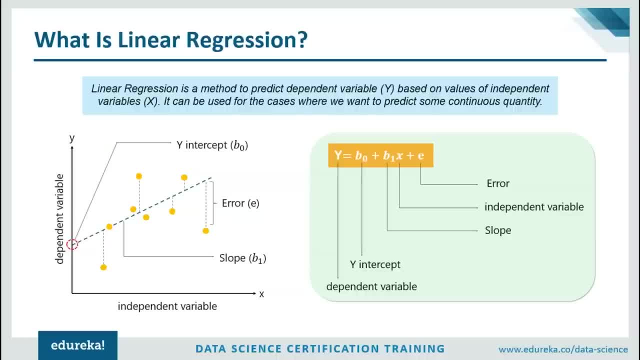 which is Y, is equal to MX plus C. So basically, the linear regression equation is represented along the same equation. All right, because this is a straight line. Let's break down this formula Now. Y over here basically stands for the dependent variable that needs to be predicted. 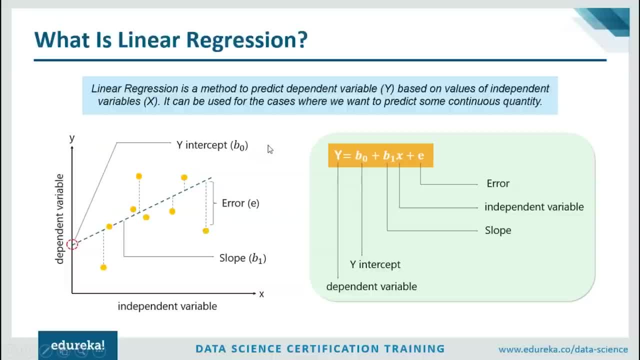 Okay, so maybe this is the stock price. now, B naught is basically the Y intercept, which is basically the point on this line which touches the y-axis. Okay, that's why it's called y-intercept. So this is our B naught over here. 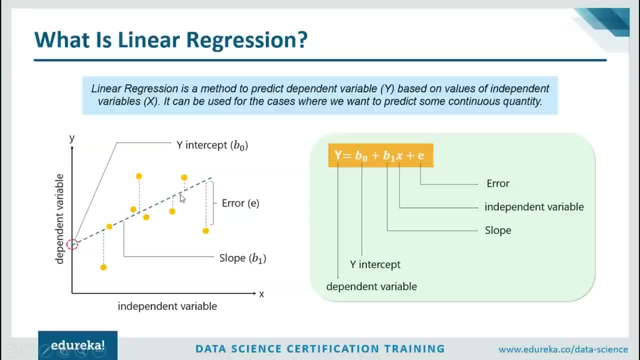 B1 is the slope of this line, this linear line, and the slope can be either negative or positive, depending on the relation between the dependent variable and the independent variable. Next we have X. X here represents the independent variable that is used to predict our result in dependent value. 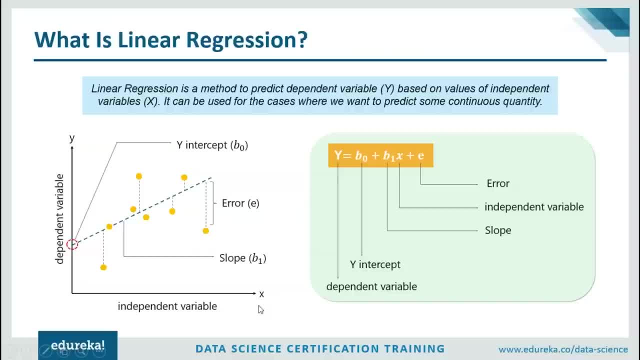 and the independent variable. next we have X, X here. It represents the independent variable that is used to predict our result in dependent value. He denotes the error in the computation. So any sort of error is denoted by E. Okay, you can see the error over here. 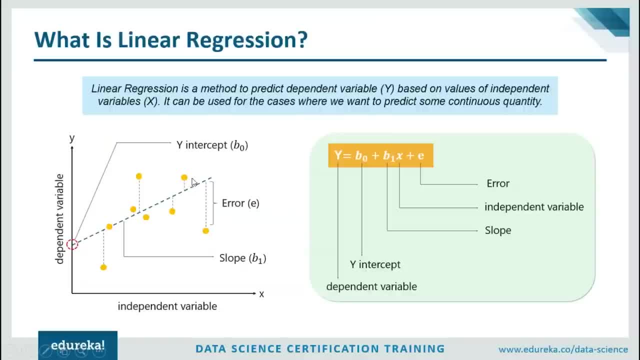 Similarly, This is the error of this data point, and so on. Okay, now that you have a basic understanding of linear regression, let's move ahead and discuss what logistic regression is. now, guys, I'm not going to go in depth about linear regression. 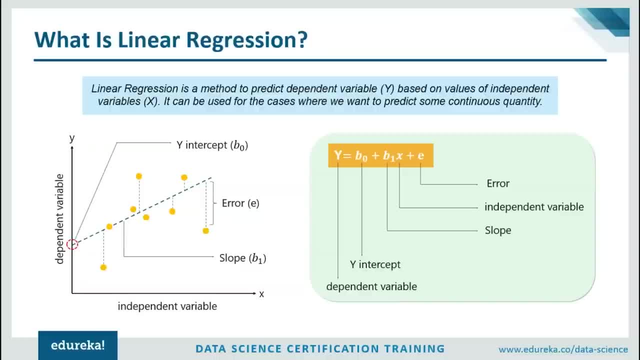 and logistic regression, because we're going to focus on the comparison between linear and logistic. Okay, but if you want to learn more about linear and logistic regression, I'm going to leave a link in the description. Y'all can check out those videos now. 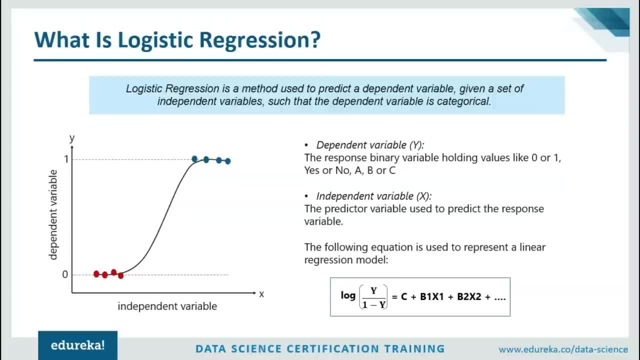 Let's look at what is logistic regression. So, guys, logistic regression is one of the basic and popular algorithms to solve a classification problem. It is named logistic because it's underlying technique is quite similar to linear regression, So logistic regression is basically a method which is used to predict a dependent variable given a set. 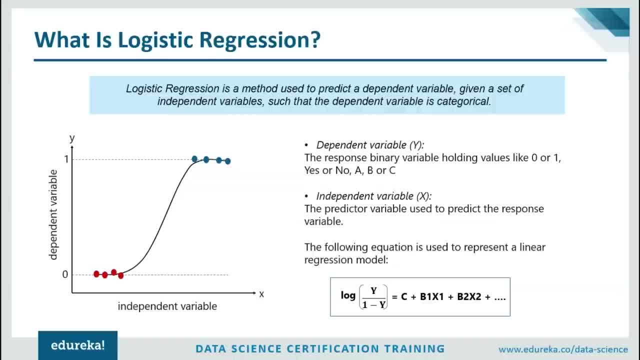 of independent variables such that the dependent variable is categorical. So, guys remember, in logistic regression the dependent variable is categorical, But when we discuss linear regression the dependent variable was always continuous. Okay, so this is one major difference between logistic and linear regression. 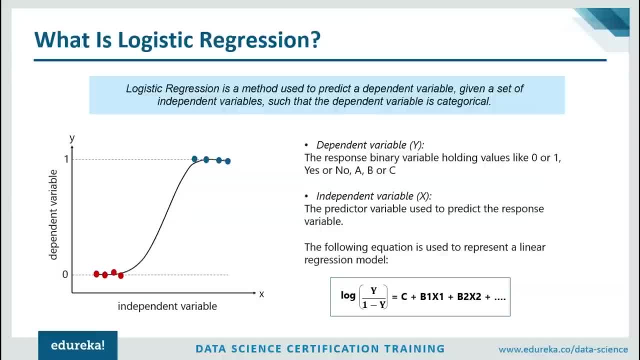 Now, what do I mean by categorical variable? So when I see categorical variable, I mean that the variable can hold values like one or zero, yes or no and so on. Okay, So basically a binary type of variable. So basically in logistic regression, 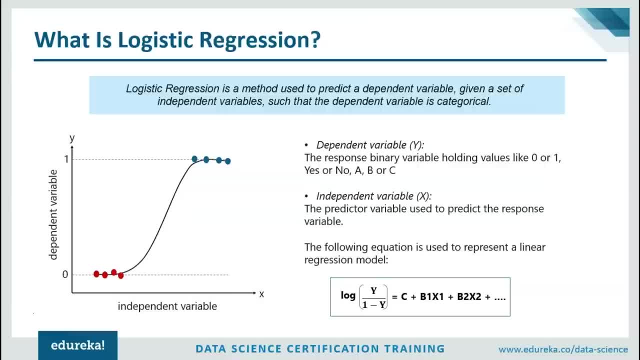 the outcome is always categorical. So when the result into outcome has only two possible values, it is always desirable to have a model that predicts the value as either 0 or 1 or as a probability score that ranges between 0 and 1. linear regression does not have 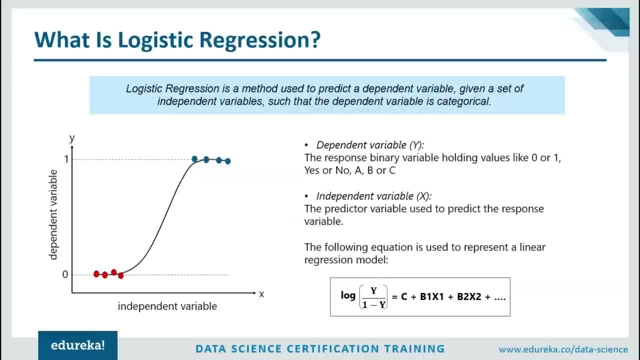 this capability? Okay, because if you use linear regression to model a binary response variable, the resulting model will not predict Y values in the range of 0 and 1. now, this is obviously because linear regression works on continuous dependent variables and not on categorical variables. 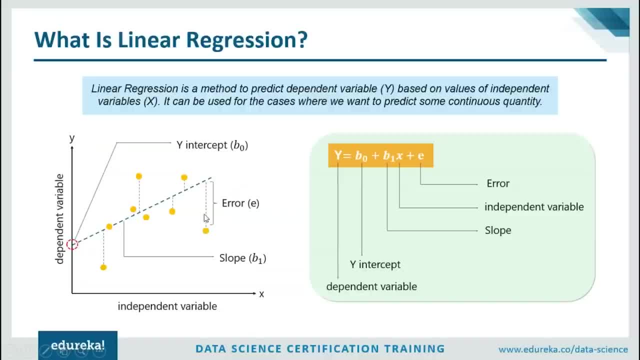 He denotes the error in the computation. So any sort of error is denoted by E. Okay, you can see the error over here. Similarly, This is the error of this data point, and so on. Okay, now that you have a basic understanding of linear regression. 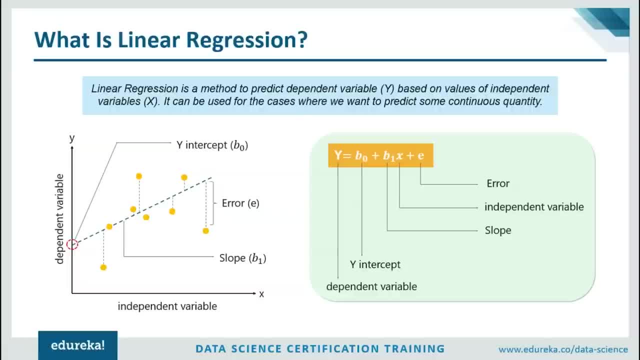 let's move ahead and discuss what logistic regression is. now, guys, I'm not going to go in depth about linear regression and logistic regression, because we're going to focus on the comparison between linear and logistic. Okay, but if you want to learn more about linear and logistic, 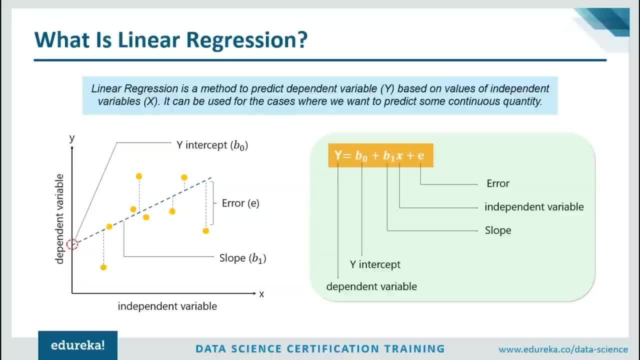 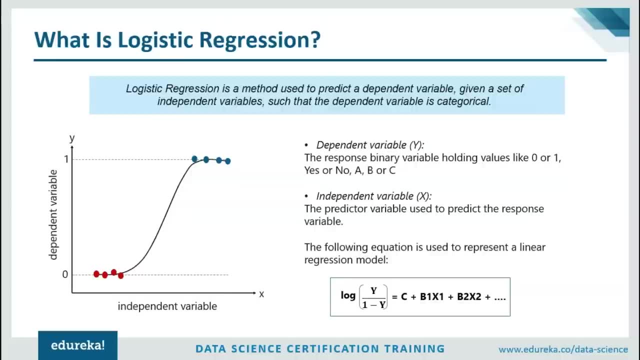 regression. I'm going to leave a link in the description. Y'all can check out those videos. now Let's look at what is logistic regression. So, guys, logistic regression is one of the basic and popular algorithms to solve a classification problem. It is named logistic because it's underlying technique is: 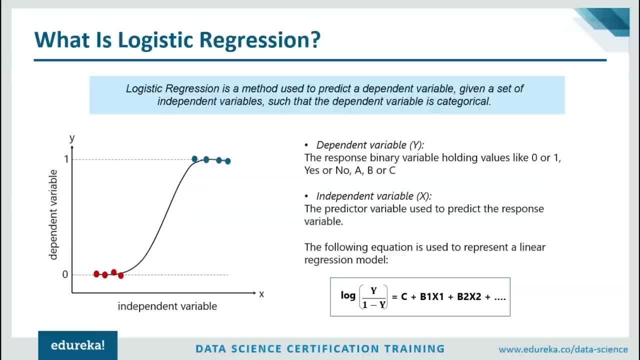 quite similar to linear regression. So logistic regression is basically a method which is used to predict a dependent variable, given a set of independent variables, such that the dependent variable is categorical. So, guys, remember, in logistic regression the dependent variable is categorical, But when we discuss linear regression, 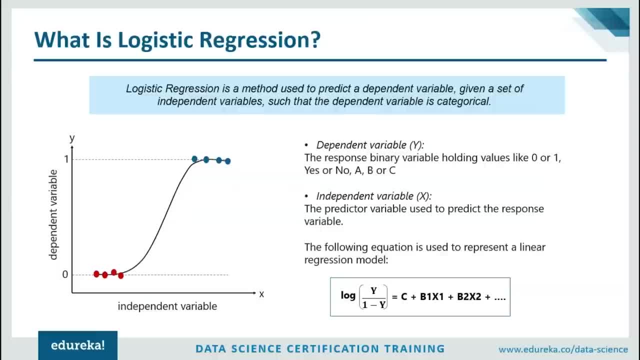 the dependent variable was always continuous. Okay, so this is one major difference between logistic and linear regression. Now, what do I mean by categorical variable? So when I see categorical variable, I mean that the variable can hold values like 1 or 0.. 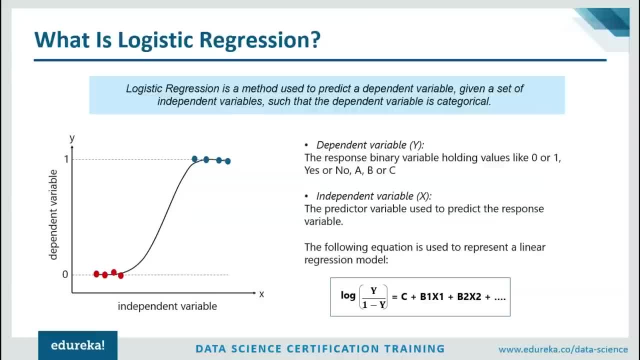 Yes or no and so on. Okay, so basically a binary type of variable. So basically, in logistic regression the outcome is always categorical. So when the resultant outcome has only two possible values, it is always desirable to have a model that predicts the value. 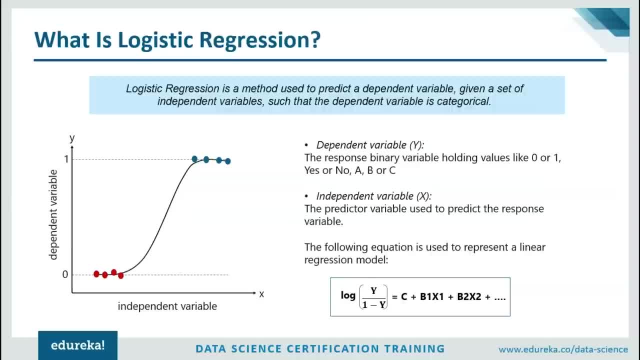 as either 0 or 1 or as a probability score that ranges between 0 and 1. linear regression does not have this capability. Okay, because if you use linear regression to model a binary response variable, the resulting model will not predict Y values. 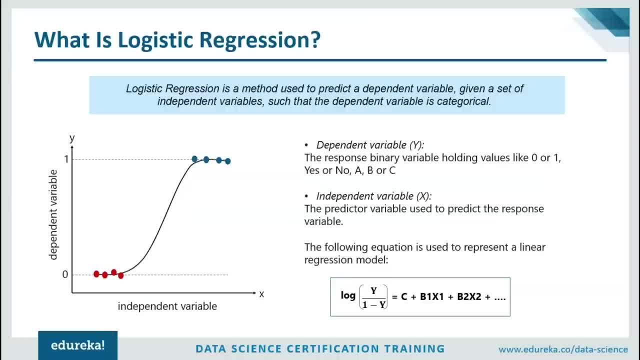 in the range of 0 and 1.. Now, this is obviously because linear regression works on continuous dependent variables and not on categorical variables. Okay, you can't expect categorical results from a linear regression model, because you're feeding it- only continuous variables. 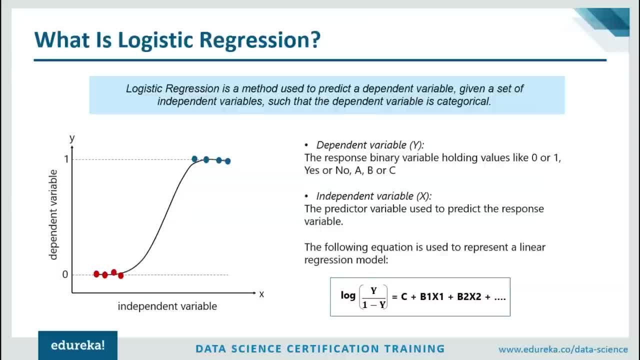 Okay, you can't expect categorical results from a linear regression model, because you're feeding it only continuous variables, correct? So, guys, that's why we make use of logistic regression. Now, the main difference, like I mentioned earlier, is the result in outcome in a linear regression model is always continuous. 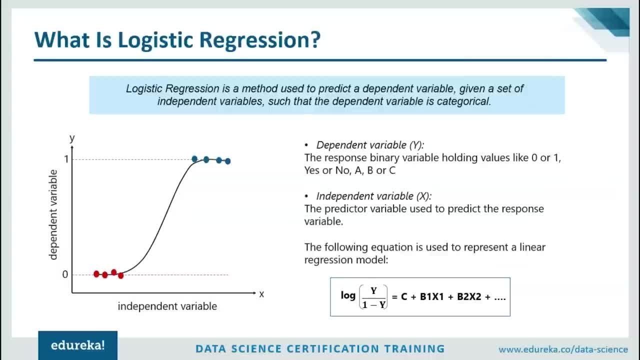 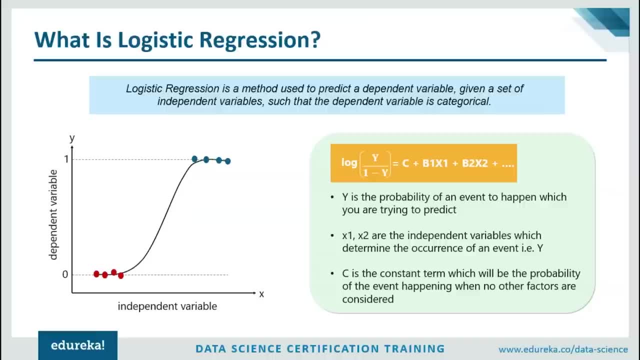 But when it comes to logistic regression, the result in outcome is categorical. Okay, Now let's discuss a little bit about the math behind logistic regression. So, guys, first of all, if you look at the graph, you can see that it's not a linear line. 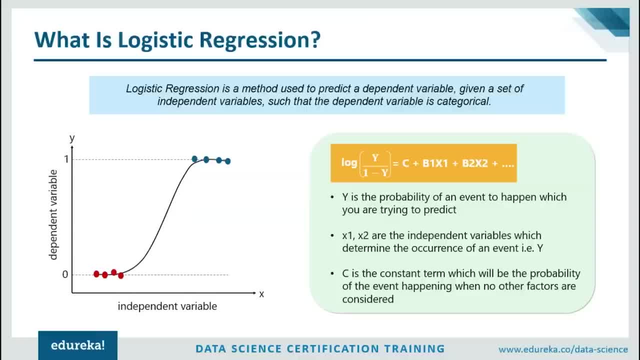 Okay, instead it is a curve. Now this curve is basically called the S curve or the sigmoid curve. The sigmoid curve Maps a relationship between the dependent and independent variable for logistic regression. Now I know that I mentioned, logistic regression only calculates the outcome as 0. 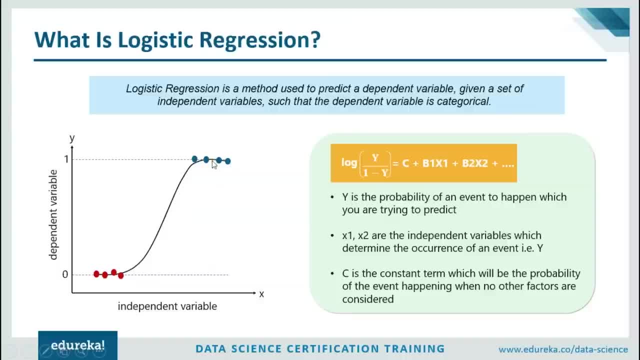 or 1.. So why do we have a curve from 0 to 1? It should be a straight line at 1 and a straight line at 0, because obviously it's outputting values as only 0 and 1. now, this is because logistic regression calculates the probability. 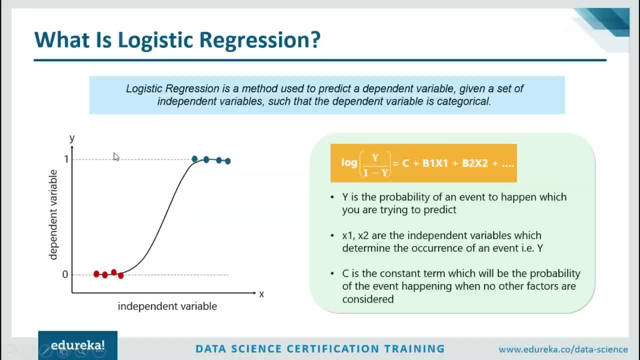 All right. So let's say that the final probability of an event occurring is 0.6.. What does this mean? Does my output belong to class number one, or does it belong to class number zero? So, guys, when such a situation occurs, we set a threshold value. 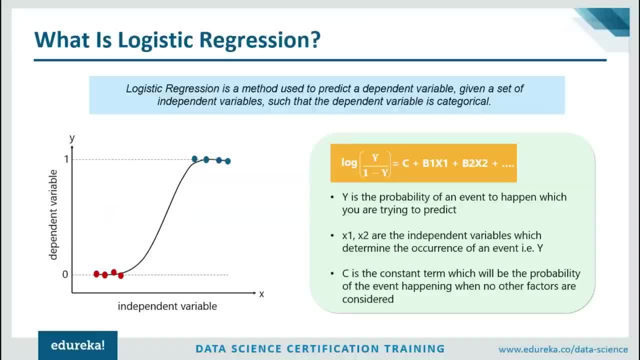 Let's say that my threshold value is 0.5.. This means that any value in the range of 0.5 to 1 is classified as 1 and any value below 0.5 is considered as 0. this way, You can easily get a binary resultant variable, which is exactly. 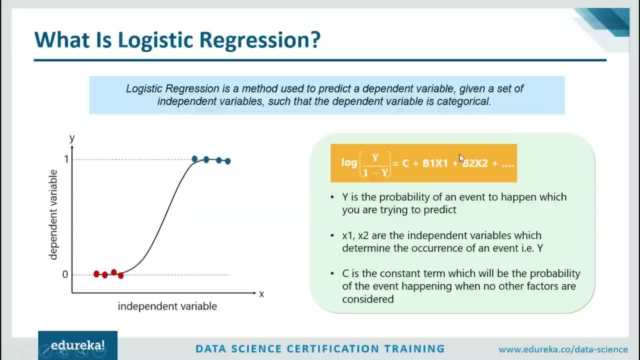 what we need when it comes to logistic regression. Now let's try to understand this equation over here. So, guys, why over here? ranges between 0 and 1.. Okay, it represents the probability Of an event to happen. Okay, so the Y value can be between 0 and 1. it can be 0.3. 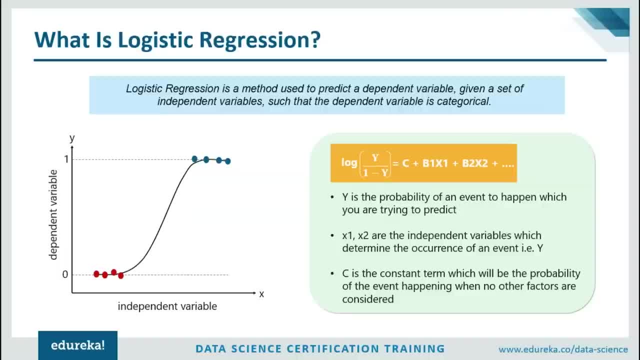 0.2, 0.6, 0.5, all of that Okay, and that's when you set a threshold value so that you can categorize the output as either 0 or 1. next We have X, 1, X, 2, X 3.. 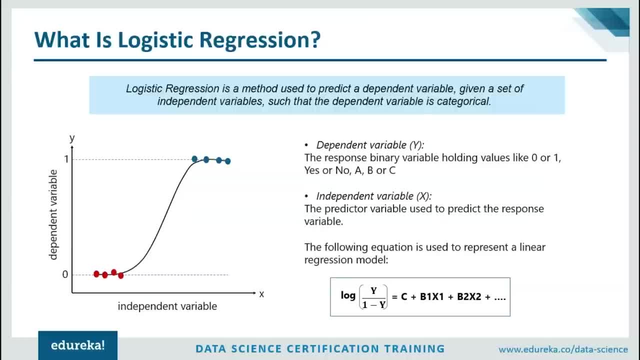 correct. So, guys, that's why we make use of logistic regression. Now, the main difference, like I mentioned earlier, is the resultant outcome. in a linear regression model is always continuous, But when it comes to logistic regression, the resultant outcome is categorical. Okay, 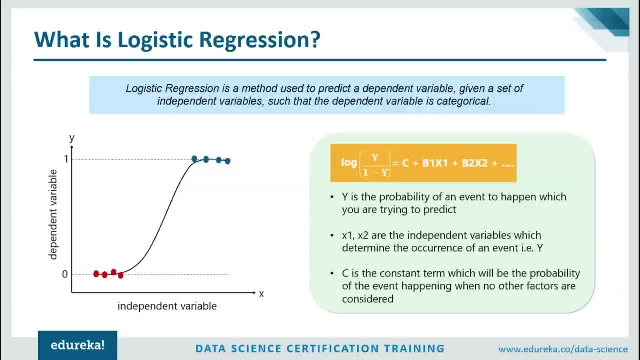 Now let's discuss a little bit about the math behind logistic regression. So, guys, first of all, if you look at the graph, you can see that it's not a linear line. Okay, instead it is a curve. Now, 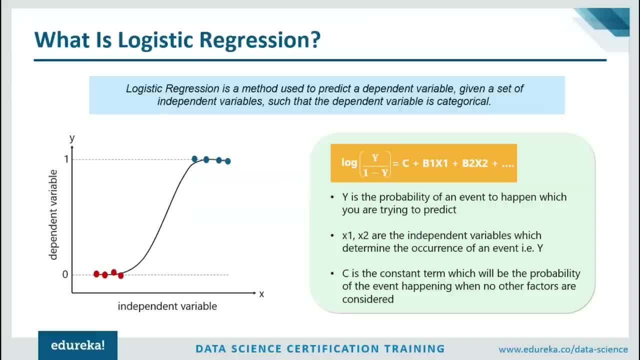 this curve is basically called the S curve or the sigmoid curve. The sigmoid curve Maps a relationship between the dependent and independent variable for logistic regression. Now I know that I mentioned logistic regression only calculates The outcome as 0 or 1.. So why do we have a curve from 0 to 1?? 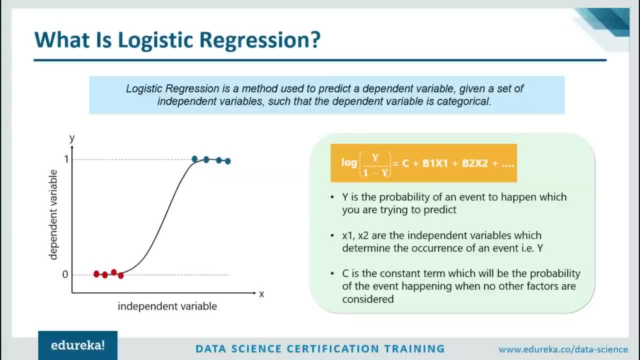 It should be a straight line at 1 and a straight line at 0, because obviously it's outputting values as only 0 and 1. now, this is because logistic regression calculates the probability. All right, So let's say that the final probability of an event occurring 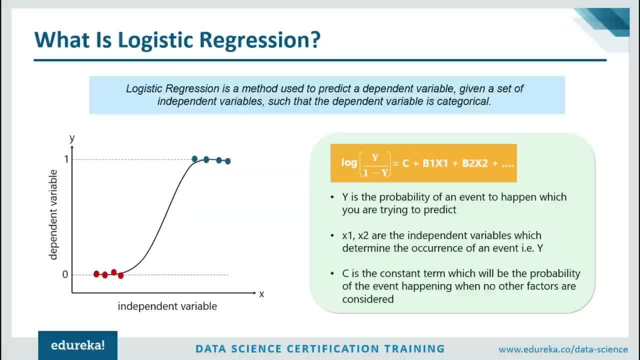 is 0.6.. What does this mean? Does my output belong to class number one, or does it belong to class number zero? So, guys, when such a situation occurs, we set a threshold value. Let's say that my threshold value is 0.5.. 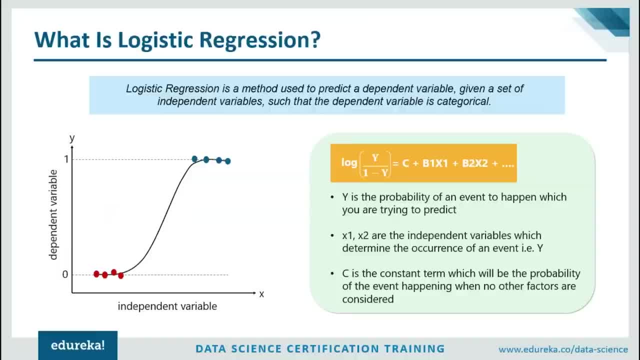 This means that any value in the range of 0.5 to 1 is classified as 1 and any value below 0.5 is considered as 0. this way, You can easily get a binary resultant variable, which is exactly what we need when it comes to logistic. 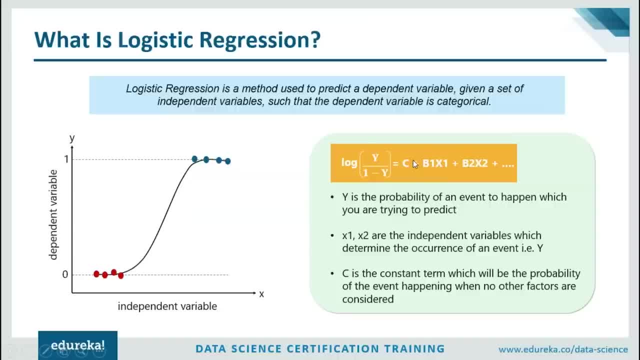 regression. Now let's try to understand this equation over here. So, guys, why over here ranges between 0 and 1?? Okay, it represents the probability of an event to happen. Okay, so the Y value can be between 0 and 1.. 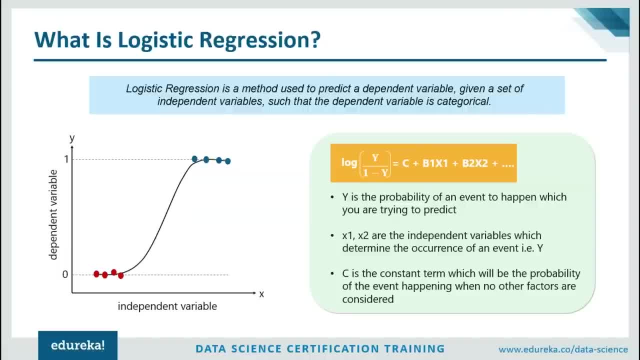 It can be 0.3, 0.2, 0.6, 0.5. all of that Okay, and that's when you set a threshold value so that you can categorize the output as either 0 or 1.. Next we have X, 1, X, 2, X, 3.. 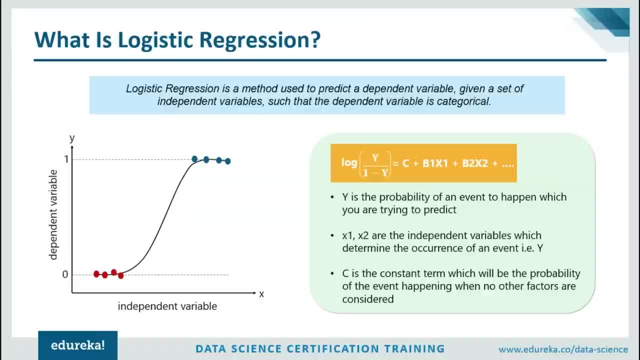 These are basically the independent variables that are used to calculate the dependent variable. now see, obviously here is the numerical constant, and B 1 and B 2 basically represent the respective coefficients of X 1, X, 2. And so on. Okay, So, guys, I'm not going to go in depth about linear. 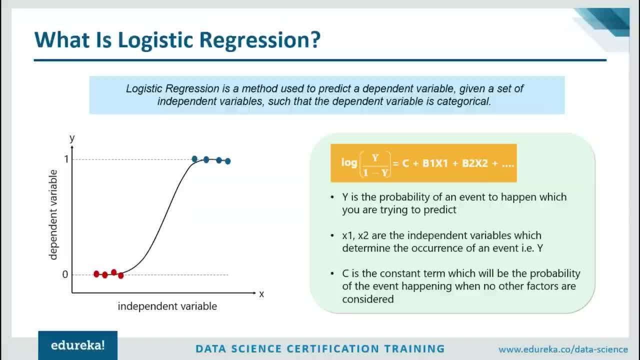 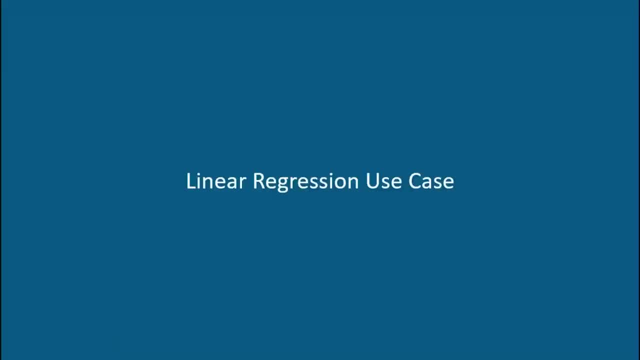 and logistic regression. I've told you all that if you want to learn more about it, I'll leave a link in the description. Y'all can go through those videos. All right, Now let's discuss a use case for linear and logistic regression. 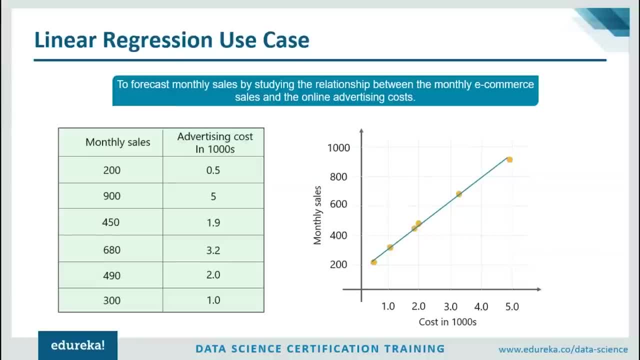 So starting with linear regression, So our problem statement here is to study the relationship between the monthly sales and the online advertising cost of some XYZ company in order to predict their sales in the upcoming months. So basically, we're going to predict the sales based on the 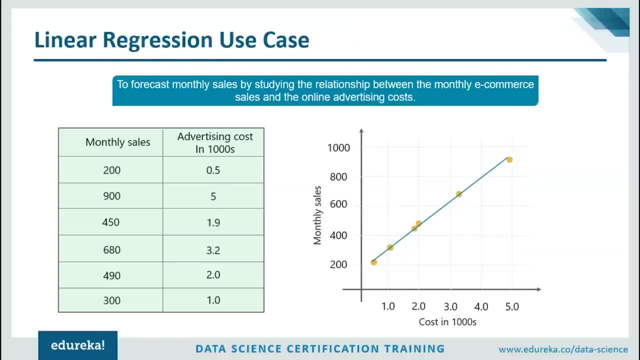 amount that they're spending on advertising. So our dependent variable becomes the number of sales. for obvious reasons, because we are going to calculate our dependent variable, which is the number of sales, and the independent variable is obviously the advertising cost. here have represented advertising costs in terms of thousand dollars. 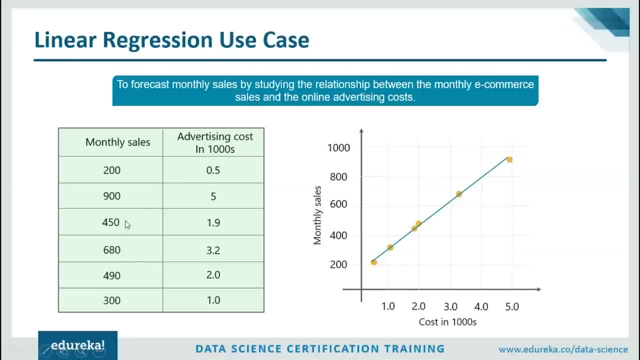 So, with the data provided in this table, if we have to plot a graph, we get a linear positive relationship between the monthly e-commerce sales And the online advertising cost. Okay, So here you can see the plot now. This is a positive correlation. 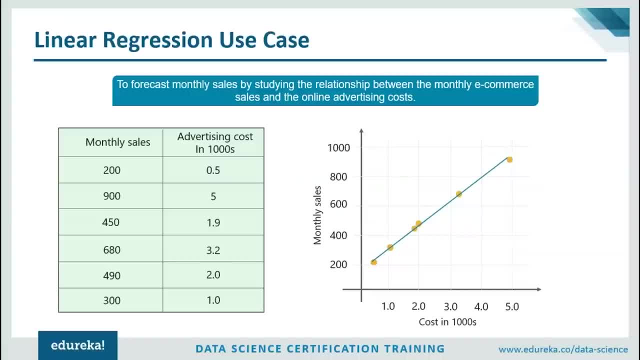 Now, when I say positive correlation, it means that the value of the dependent variable Y, which is basically the number of sales, increases with the value of the independent variable. Okay, That's why you see the line going up. This is called a positive slope or a positive correlation, meaning: 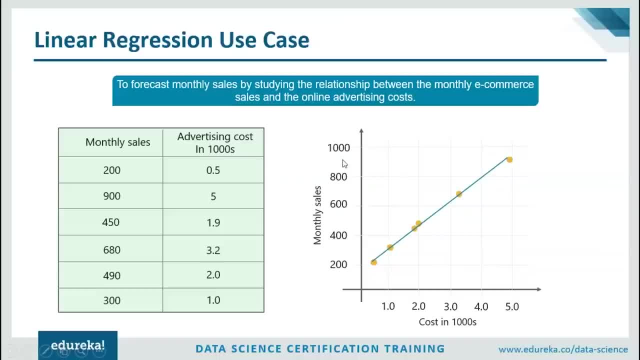 that if you increase the advertising cost, your monthly sales will also increase. So you can use this To predict your future sales. So you know that now, if you keep increasing your advertising costs, your monthly sales will also increase. so, guys, linear regression has a lot of applications in the business sector. 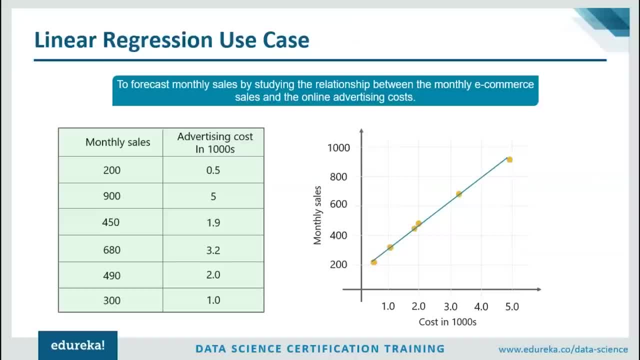 It is used to forecast sales, to perform risk analysis, measure the profit probability, and so on. Now let's take a look at a use case for logistic regression. So, guys, our problem statement here is to predict if a student will get admitted to a school based on his CGPA. 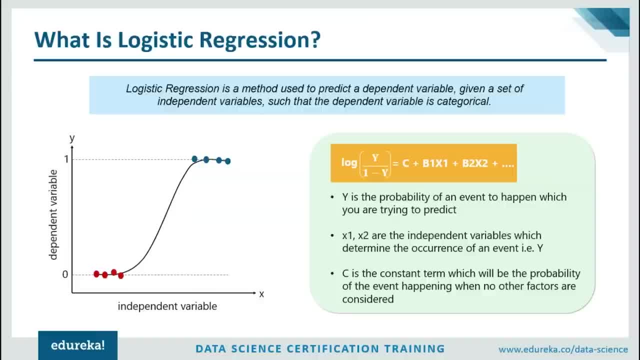 These are basically the independent variables that are used to calculate the dependent variable. Now see, obviously here is the numerical constant, and B 1 and B 2 basically represent the respective constant Coefficient of X 1, X 2, and so on. Okay, 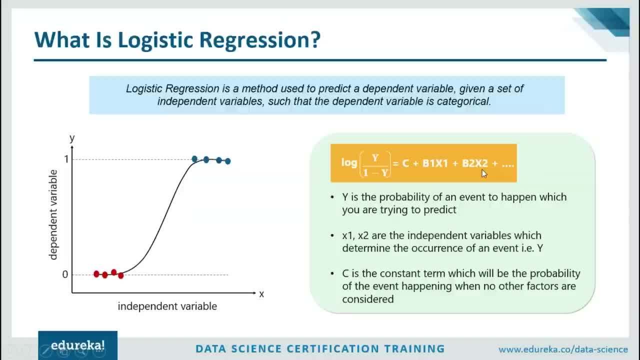 So, guys, I'm not going to go in depth about linear and logistic regression. I've told you all that if you want to learn more about it, I'll leave a link in the description. Y'all can go through those videos, All right. 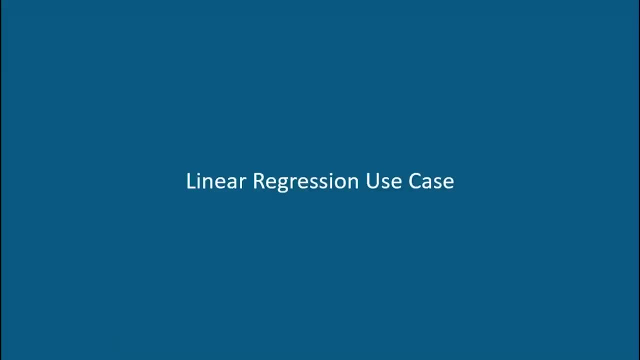 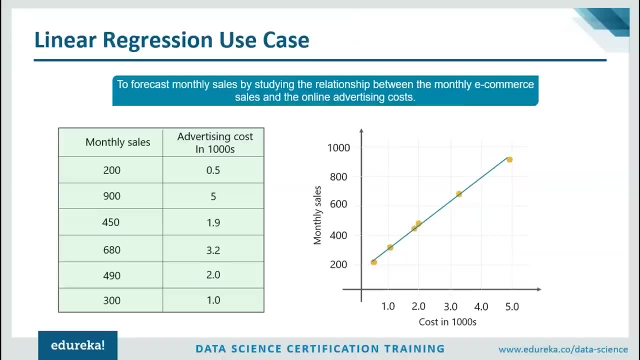 Now let's discuss a use case for linear and logistic regression. So starting with linear regression. So our problem statement here is to study the relationship between the monthly sales and the online advertising cost of some XYZ company in order to predict their sales in the upcoming months. 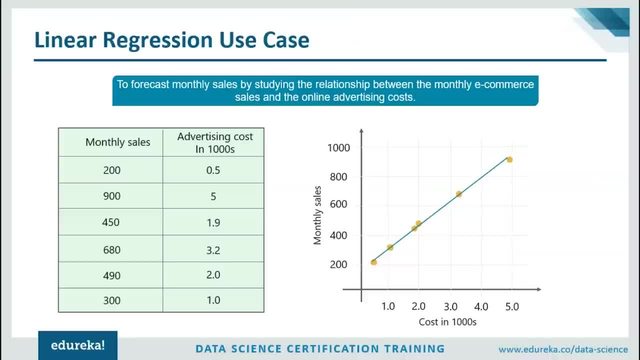 So basically, we're going to predict the sales based on the amount that they're spending on advertising. So our dependent variable becomes the number of sales. for obvious reasons, because we are going to calculate our dependent variable, which is the number of sales, and the independent variable is: 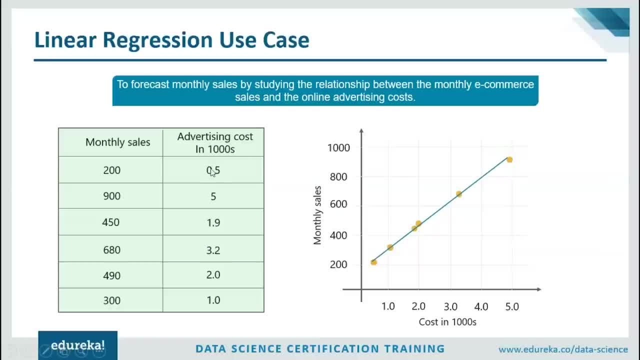 obviously the advertising cost here have represented advertising costs in terms of thousand dollars. So with the data provided in the stable, if we have to plot a graph, we get a linear positive relationship between the monthly e-commerce sales and the online advertising cost. Okay, So here you can see the plot now. 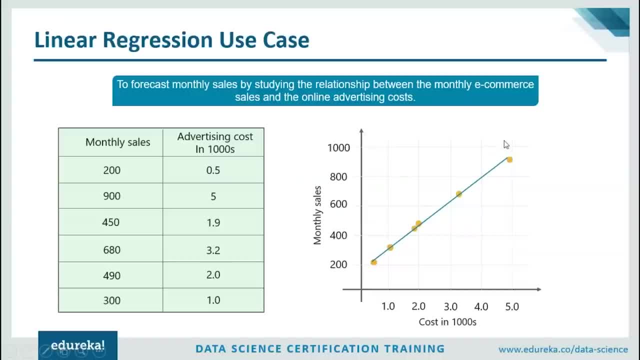 This is a positive correlation. Now, when I say positive correlation, it means that the value of the dependent variable Y, which is basically the number of sales, increases with the value of the independent variable. Okay, That's why you see the line going up. 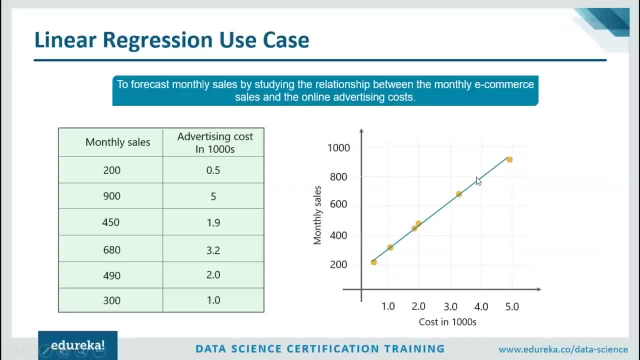 This is called a positive slope or a positive correlation, meaning that if you increase the advertising cost, your monthly sales will also increase. So you can use this plot to predict your future sales. So you know that now: if you keep increasing your advertising costs, your monthly sales will also increase. 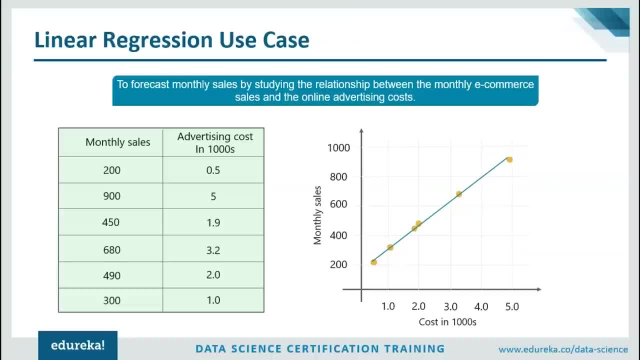 So, guys, linear regression has a lot of applications in the business sector. It is used to forecast sales, to perform risk analysis, measure the profit probability, and so on. Now let's take a look at a use case for logistic regression. So, guys, our problem statement here is to predict if a student 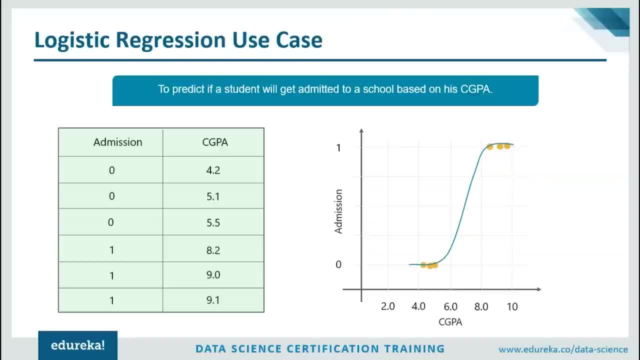 will get admitted to a school based on his CGPA. So if you look at our data set, it contains two variables: the CGPA and the admission variable. So, guys, X over here indicates the CGPA and Y indicates whether these students will get an admission in college. 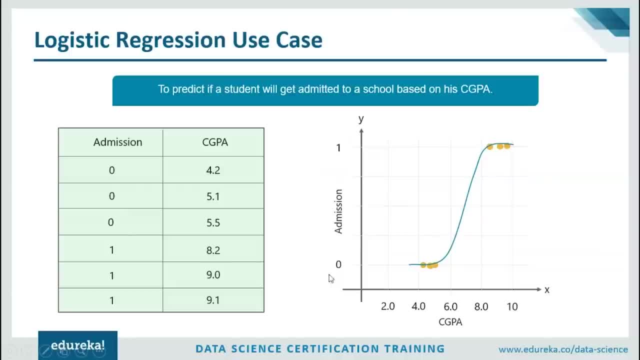 Okay. So one here will mean that you've got an admission, and zero means no, admit. Okay. Now here the logistic regression will help assess what level of CGPA leads to admission in a college. So the logistic model is trained In such a way that the students with a CGPA of 6 and above 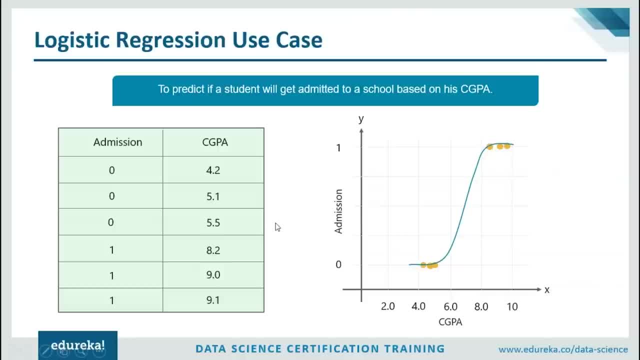 get admission. Okay. hence Y equals to 1. but if the CGPA is below 6, they don't get an admission. Okay, that's when Y equals to 0.. So the students classified in the group Y equal to 1 will get. 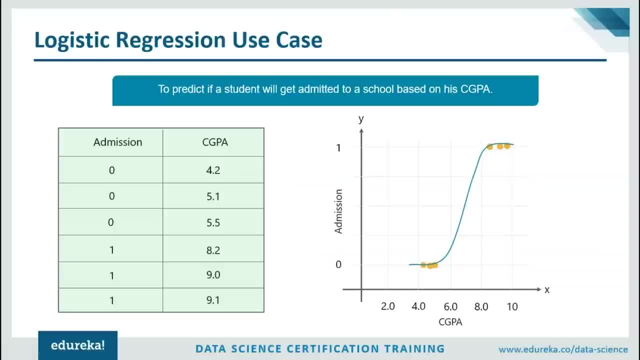 an admission, Whereas the students in the group Y, equal to 0, will not get an admission. Now, guys, in a similar manner, logistic regression is used to solve n number of complex classification problems. It is used in the cybersecurity domain To detect fraudulent customers. 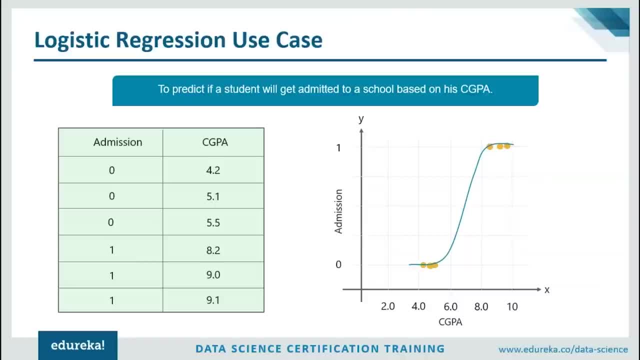 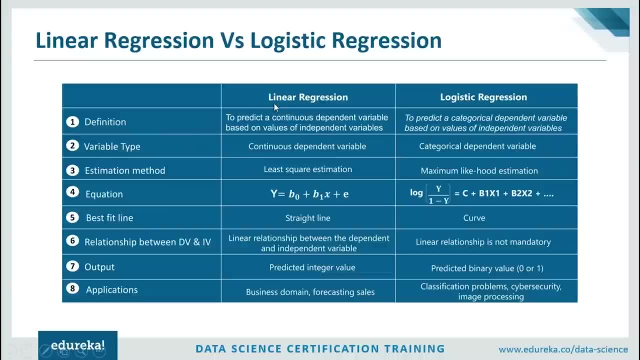 It is used in image classification and a lot other classification problems. Okay, Now let's try to sum up our entire session and let's compare the two models. So first of all, let's look at the definition of linear regression and logistic regression. 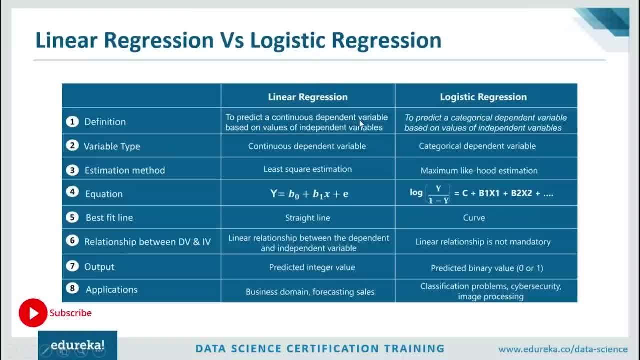 So the main aim of linear regression is to predict a continuous dependent variable based on the values of the independent variables. But when it comes to logistic regression, the aim is to predict a categorical dependent variable Variable based on the values of independent variables. These are the main aim of each of these models. 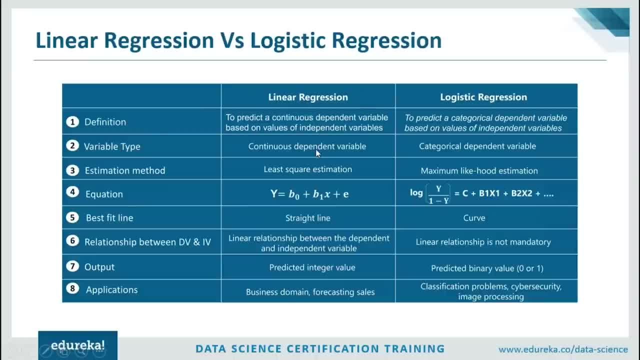 Now let's look at the variable type. now, in linear regression, The dependent variable is always continuous. All right, this is very important to remember, because this is the main objective of linear regression. Okay, it makes use of continuous dependent variables to predict continuous values. 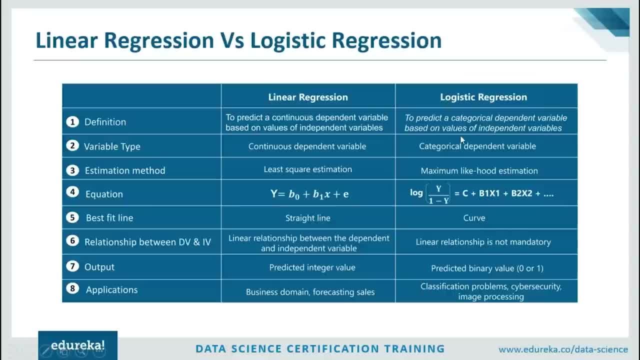 Similarly, when it comes to logistic regression, you're going to use categorical dependent variable to predict a categorical value. All right, Now let's look at the estimation method. So, guys, linear regression is based on the least square estimation, which basically says that the regression 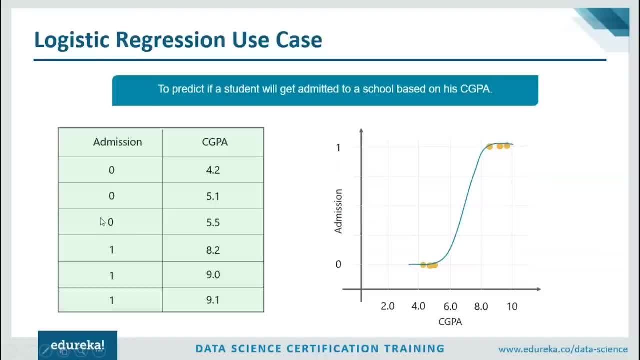 So if you look at our data set, it contains two variables: the CGPA and the admission variable. so, guys, X over here indicates the CGPA and Y indicates whether these students will get an admission in college. Okay, so one here will mean that you've got an admission and 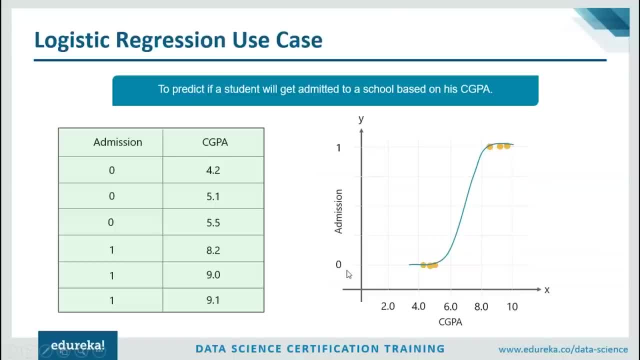 zero means no admit. Okay, Now here, the logistic regression will help assess what level of CGPA leads to admission in a college. So the logistic model is trained in such a way that the students' with a CGPA of 6 and above get admission. 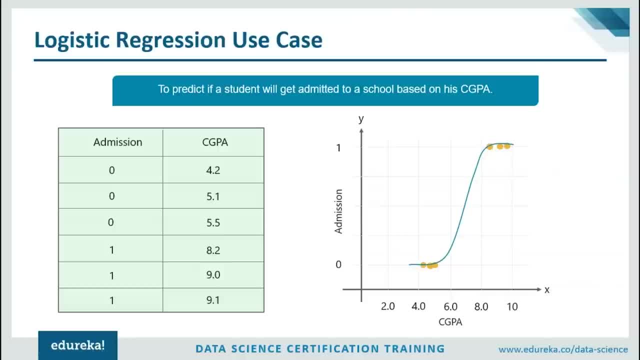 Okay, hence Y equals to 1, but if the CGPA is below 6, they don't get an admission. Okay, that's when Y equals to 0. so the students classified in the group Y equal to 1 will get an admission, whereas the students 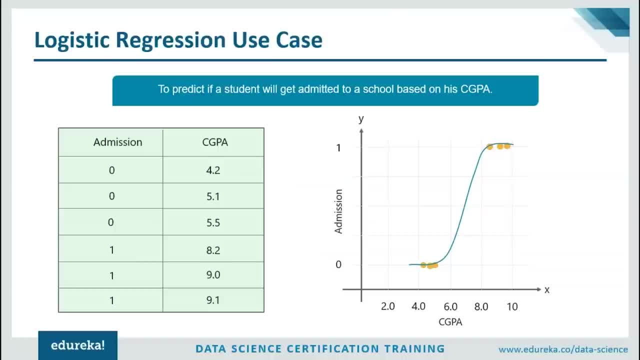 in the group Y equal to 0 will not get an admission. now, guys. in a similar manner, logistic regression is used to solve n number of complex classification problems. It is used in the cyber security domain to detect fraudulent customers. It is used in image classification and a lot other classification. 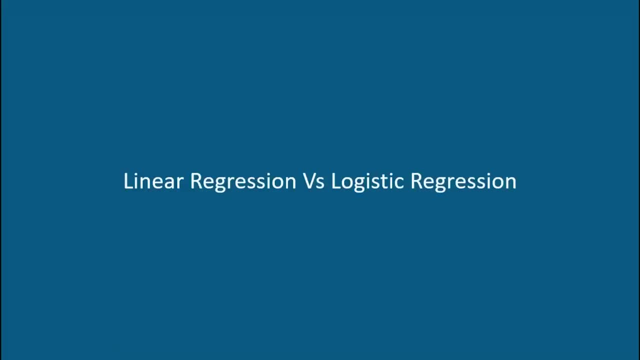 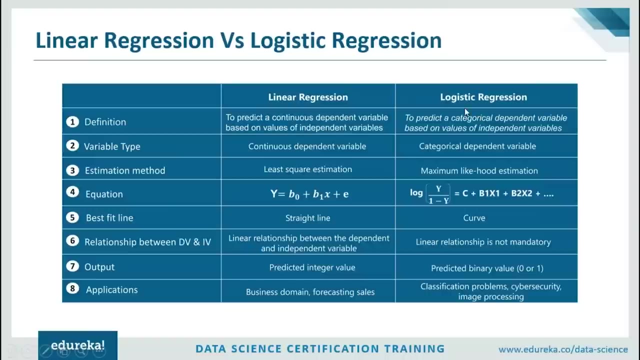 problems. Okay, Now let's try to sum up our entire session and let's compare the two models. So first of all, let's look at the definition of linear regression and logistic regression. So the main aim of linear regression is to predict a continuous 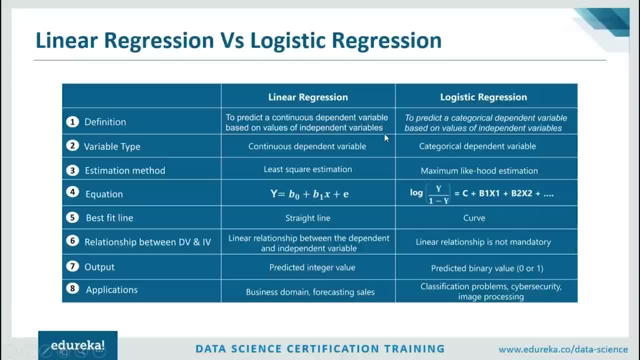 dependent variable based on the values of the independent variables. but when it comes to logistic regression, the aim is to predict a categorical dependent variable based on the values of independent variables. These are the main aim of each of these models. Now let's look at the variable type now in linear regression. 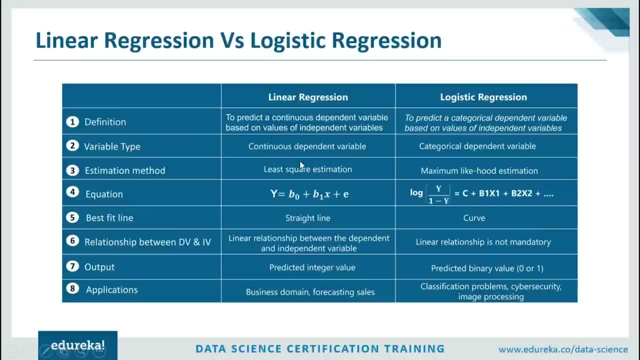 The dependent variable is always continuous. All right, This is very important to remember, because this is the main objective of linear regression. Okay, it makes use of continuous dependent variables to predict continuous values. Similarly, when it comes to logistic regression, you're going? 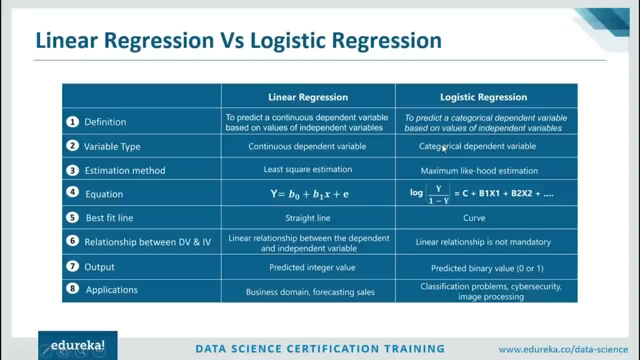 to use categorical dependent variable to predict a categorical value. All right, Now let's look at the estimation Method. so, guys, linear regression is based on the least square estimation, which basically says that the regression coefficient should be chosen in such a way that it minimizes the sum of the 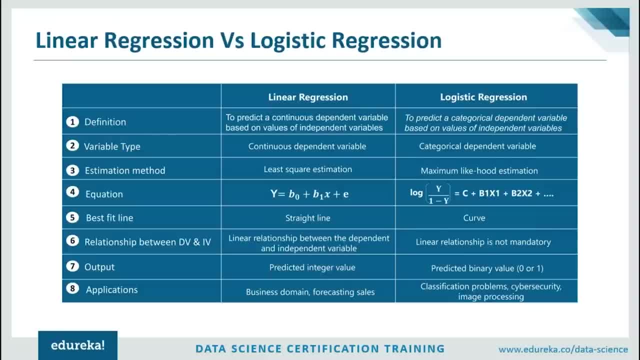 coefficient should be chosen in such a way that it minimizes the sum of the square distance of each observed response. Okay Now, this is in-depth about linear regression, So that's why I'm going to leave a link in the description now. logistic regression, on the other hand, is based on maximum. 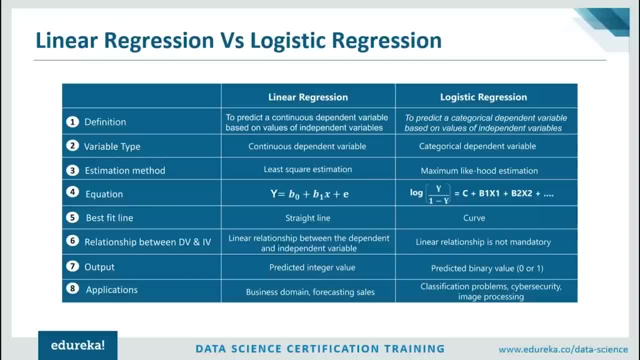 likelihood estimation. Okay, this basically says that the coefficients should be chosen in such a way that it maximizes the probability of Y given some value of X. next is the equation earlier We discuss this equation where for linear regression we have Y is equal to B, naught plus B, 1 into X plus E. 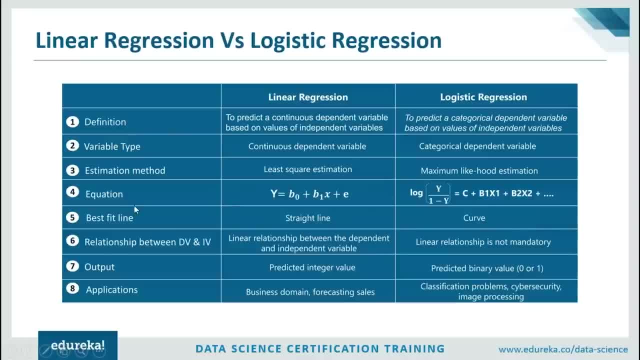 Okay, Similarly, this is the equation for logistic regression. So the next difference is the best fit line. So, guys, linear regression aims at finding the best fitting straight line, which is also called the regression line. All right, But when it comes to logistic regression, 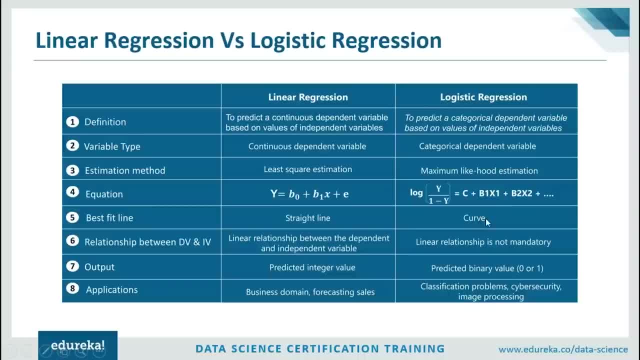 if you try and map the relationship between the dependent and independent variable, you're going to get a curve, which is also known as a sigmoid curve. All right, So in linear regression, the relationship between the dependent and independent variable is represented using a straight line. 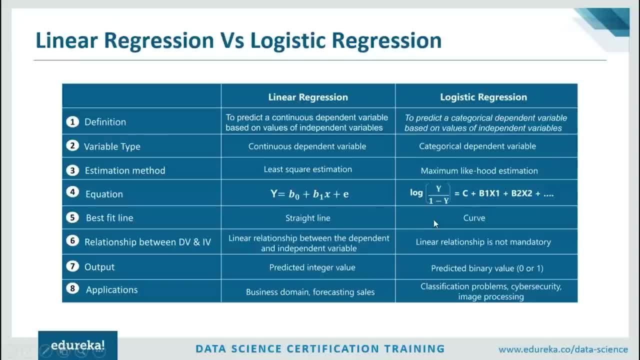 But when it comes to logistic regression, the relationship between the dependent and independent variable is represented using a sigmoid curve. Now let's look at the relationship between dependent and independent variable. Now, when it comes to linear regression, there has to be a linear relationship between the two. 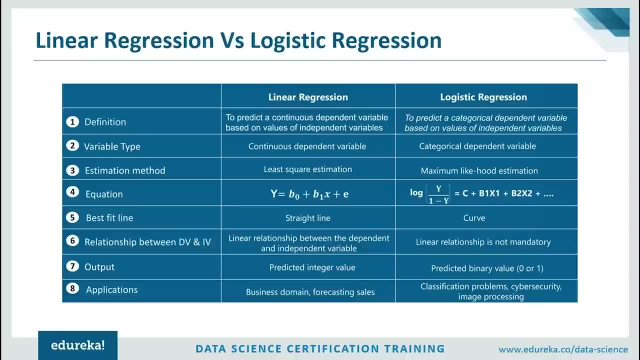 So when I say linear, I mean that the variables have to vary linearly. Okay, that's how the straight line is formed in the first place. All right, when it comes to logistic regression, it's not necessary to have a linear relationship. 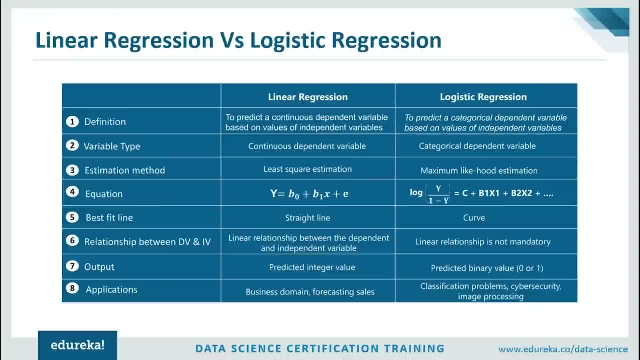 Now, the output of linear regression is always going to be a predicted integer value or basically a continuous value. So when it comes to logistic regression, the output has to be a binary value. Okay, so it should either be class A or class B, or should be 0 or 1, something like that. 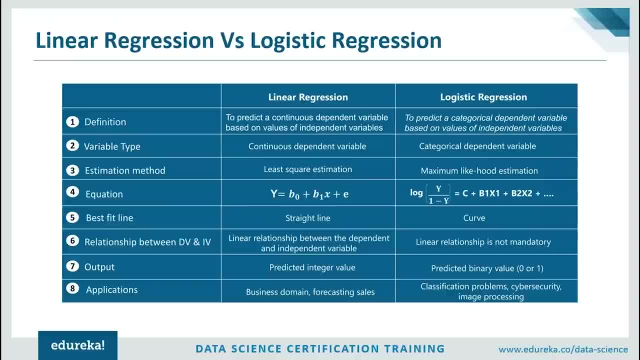 Finally, we have applications now. linear regression is mainly used to predict outcomes like the expected number of sales, and you know it's always used to predict some continuous value, All right. but when it comes to logistic regression, it's mainly used in classification. 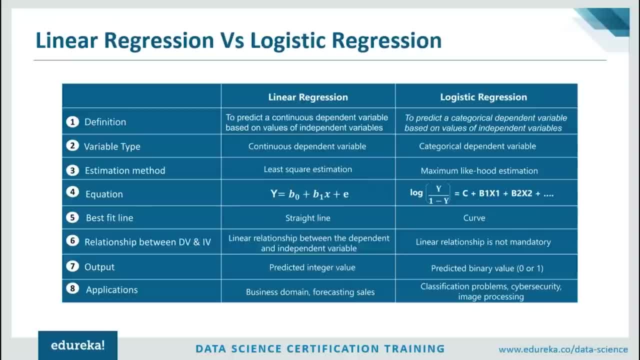 square distance of each observed response. Okay, Now, this is in-depth about linear regression, So that's why I'm going to leave a link in the description Now. logistic regression, on the other hand, is based on maximum likelihood estimation. Okay, This basically says that the coefficients should be chosen in. 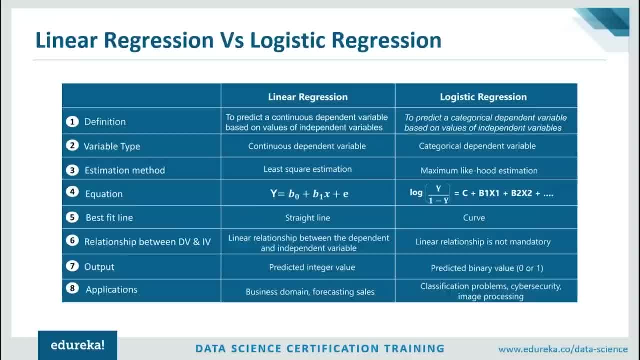 such a way that it maximizes the probability of Y given some value of X. next is the equation- earlier We discussed this equation- where for linear regression we have Y is equal to B, naught plus B 1 into X plus E. Okay, Similarly, this is the equation for logistic regression. 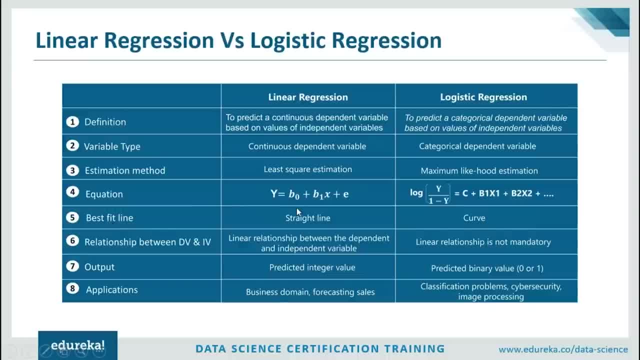 So the next difference is the best fit line. So, guys, linear regression aims at finding the best fitting straight line, which is also called the regression line. All right, but when it comes to logistic regression, right If you try and map the relationship between the dependent 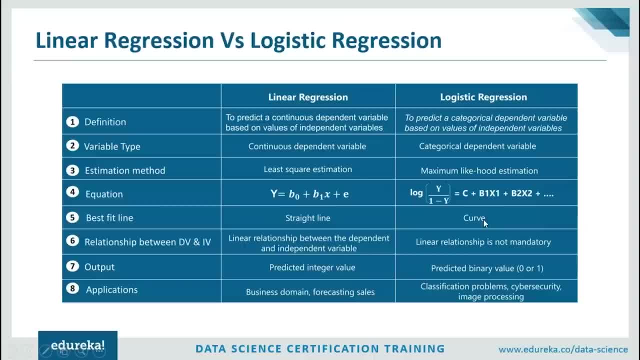 and independent variable, you're going to get a curve, which is also known as a sigmoid curve. All right. So in linear regression, the relationship between the dependent and independent variable is represented using a straight line, But when it comes to logistic regression, the relationship 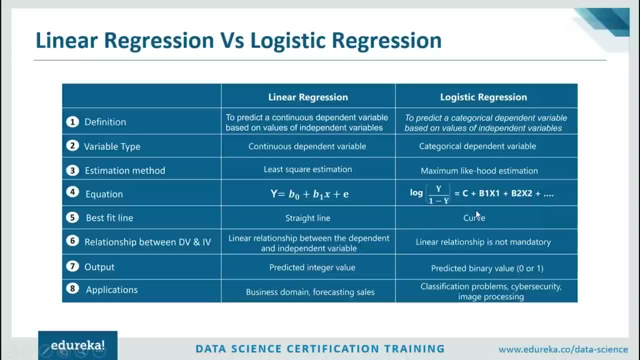 between the dependent and independent variable is represented using a sigmoid curve. Now let's look at the relationship between dependent and independent variable. Now, when it comes to linear regression, there has to be a linear relationship between the two. So when I say linear, 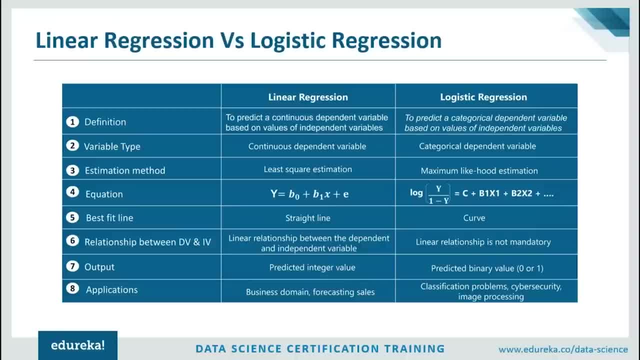 I mean that the variables have to vary linearly. Okay, that's how the straight line is formed in the first place. All right, when it comes to logistic regression, it's not necessary to have a linear relationship. Now, the output of linear regression is always going. 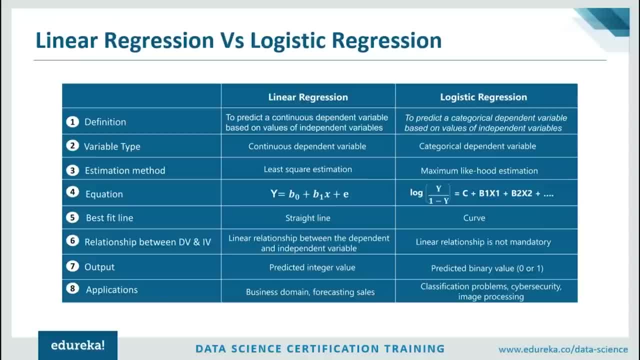 to be a predicted integer value or basically a continuous value. So when it comes to logistic regression, the output has to be a binary value. Okay, so it should either be class A or class B, or it should be 0 or 1, something like that. 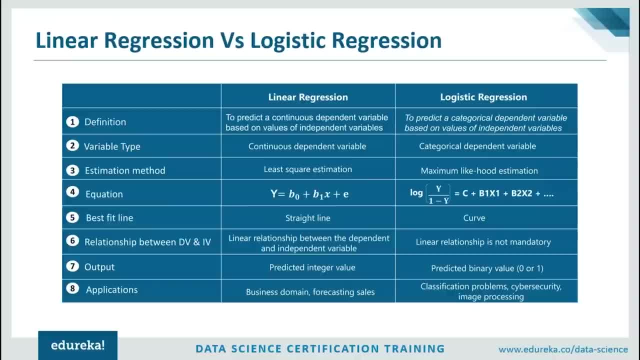 Finally, we have applications now. linear regression is mainly used to predict outcomes like the expected number of sales, and you know it's always used to predict some continuous value, All right. but when it comes to logistic regression, it's mainly used in classification.